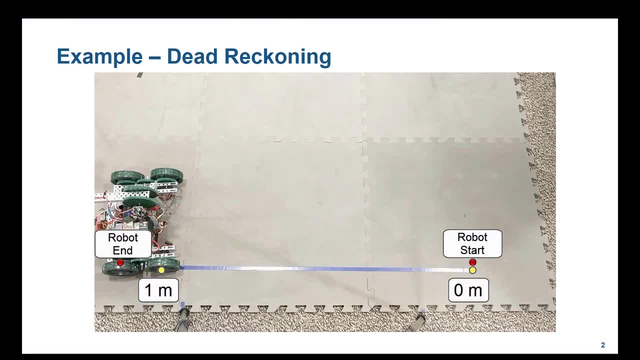 These kinds of processes, where we use the distance traveled by the robot to determine its position, is called dead reckoning. In general, this falls under the problem of knowing where the robot is, and this is called localization. One possible way to do this is to use what are called encoder. 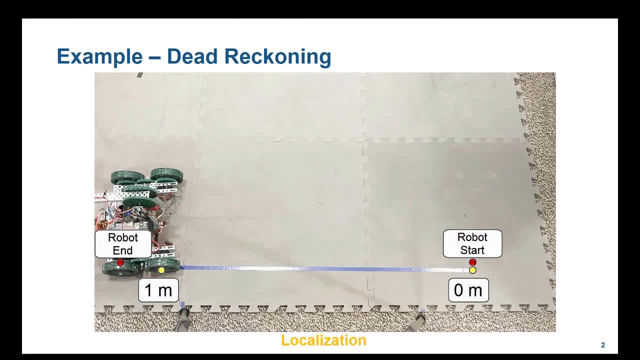 sensors to compute the number of rotations of the wheel to determine the distance traveled. Other popular ways to achieve localization are to use other sensors such as a GPS, an IMU, a camera, LIDAR, etc. In our example, we will stick to using the encoder sensors. 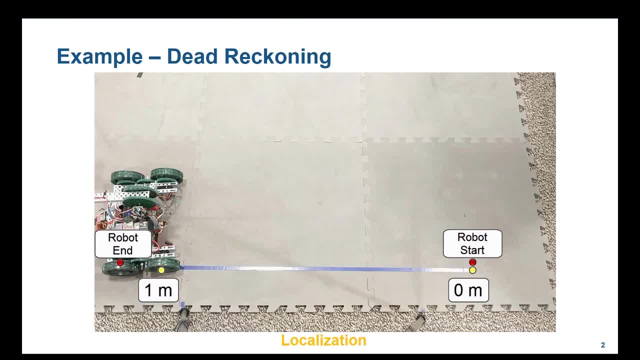 to implement the dead reckoning algorithm, with the final goal being to move the robot in a straight line for 1 meter. We will use Simulink to do this. But first, what is Simulink? Let's look at this from a higher aspect. 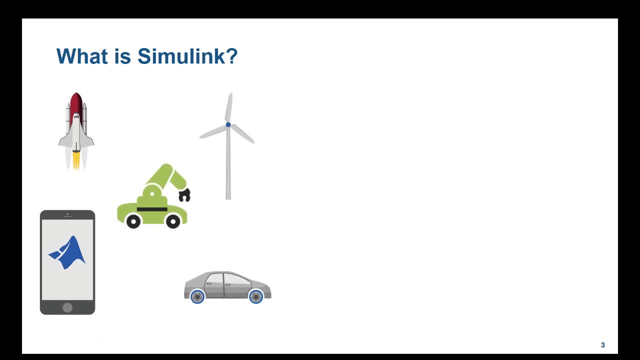 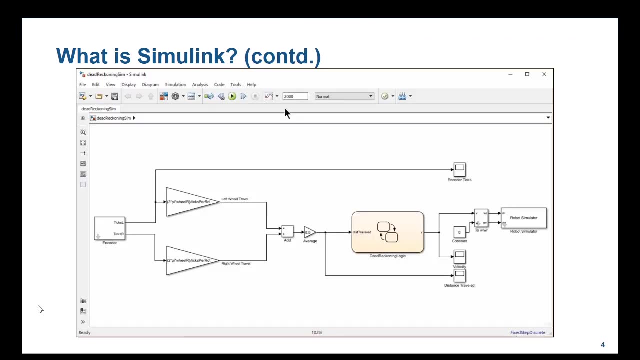 level. many engineering applications such as space communications, automotive, energy and robotics usually involve tasks that require you to write a lot of code to solve a problem. in simulink, we express this problem as a block diagram using what are called models. models represent various components in our system. in our case, where we want to model the system of equations for a differential 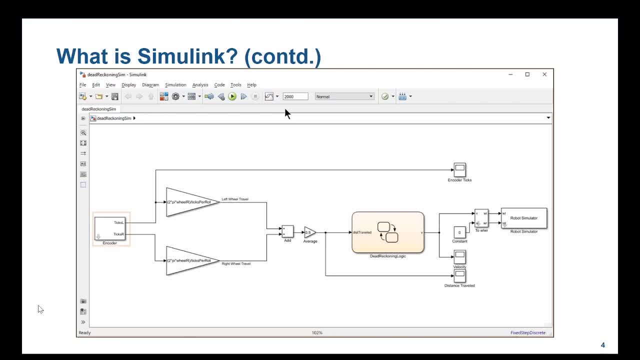 drive robot and the logic to move it. here are the input sensors, the calculations, the robot logic and a way to visualize the simulation. once we have built the model, we run our simulation. checking the results. we see the robot position and the fact that it moves for one meter. 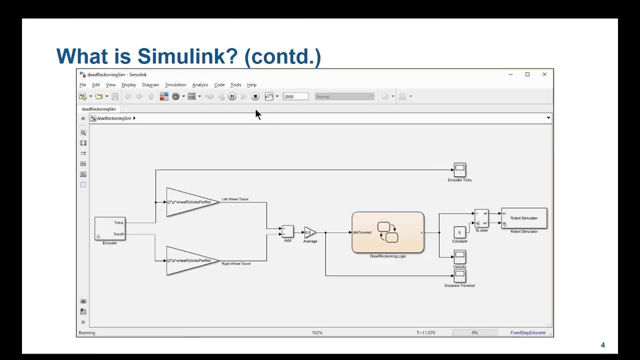 we also see time traces of various variables plotted versus time, such as distance traveled and velocity. this is because in simulink, all our simulations are time dependent. using simulations like this, you can explore what-if scenarios that are impractical to perform in real life. but simulation can only take you so far. at some point you need to be able. 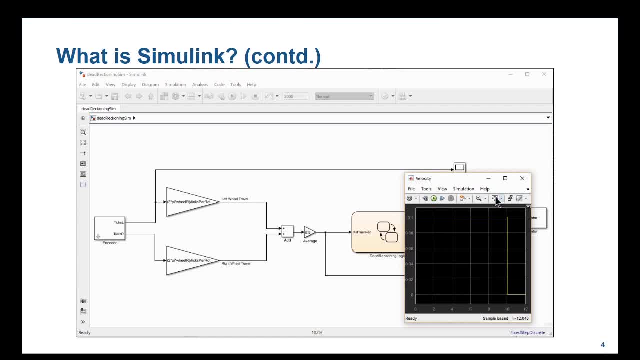 to perform these tests with the real hardware. this is also possible in simulink using hardware support packages. we will talk about hardware support packages later on in this video. okay, now that we know at a high level what simulink is, let's go back to our original problem of moving. 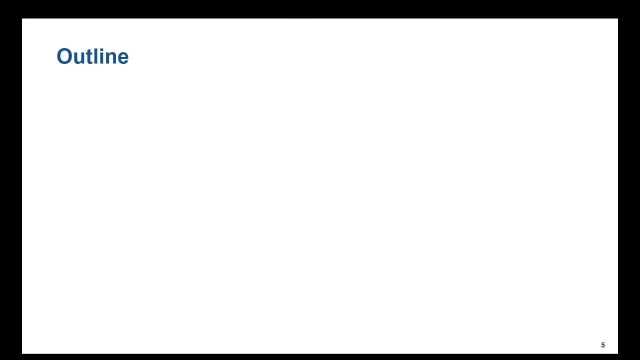 the robot for a prescribed distance. to understand how to do this, we will talk about the basics of encoder sensors. understanding the problems we will be discussing today are the following: some of the how to calculate distance using encoder sensors: implementing a dead reckoning algorithm. given a prescribed distance to travel, how to move the robot by that. 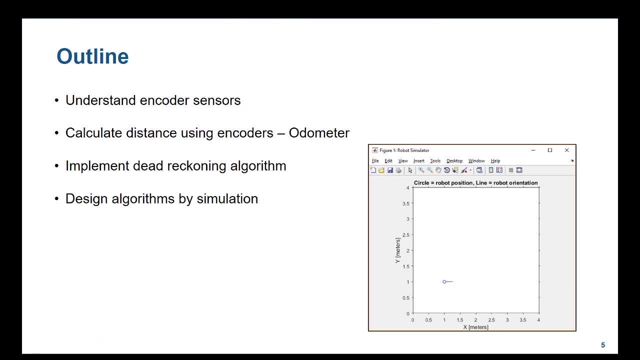 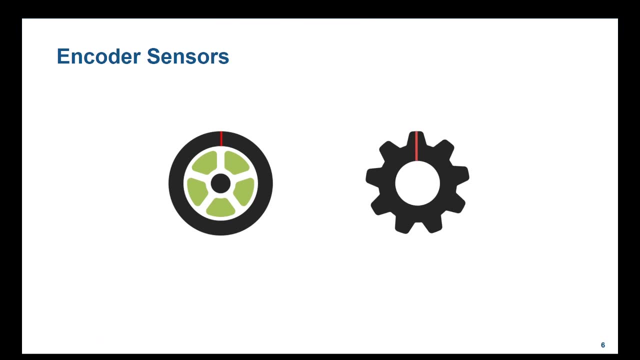 much distance. we will then test our dead reckoning algorithm using simulation and finally we will look at verifying the algorithm on an example hardware. first, let's talk about the encoder sensor. basics assume that we have a wheel like this. an encoder is a device that is connected to the wheel motor shaft. now 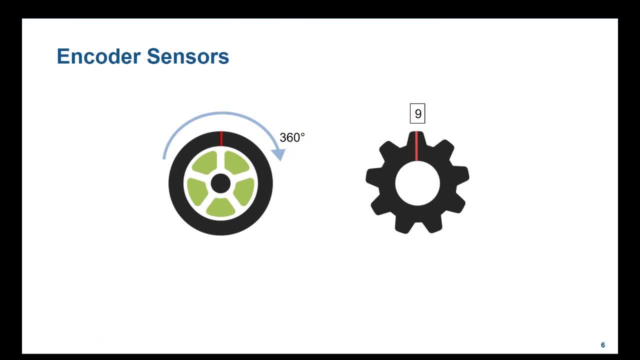 if we rotate this wheel by one full revolution, which is 360 degrees, the encoder counts discrete number of ticks corresponding to the rotation. in our case, nine ticks by the encoder means one full rotation or 360 degrees. we can use this information to determine the number of wheel rotations. 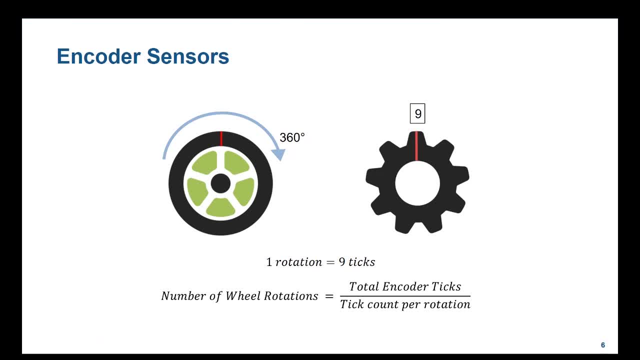 you know, we count the total number of encoder ticks and divide that by the tick count per rotation value. in our example, this is nine. in reality, this could be found on the manufacturer data sheet of the encoder. now we know how to compute the number of wheel rotations with an encoder, but how is this useful? 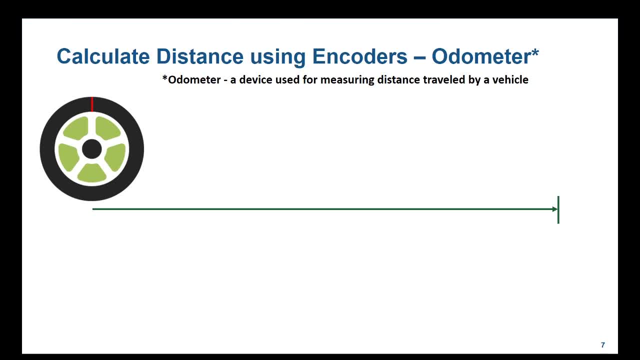 to calculate distance. a device that is used to measure the distance traveled is also called an odometer. so let's see how to use encoders to build a moment. let's stick our wheel again this time when we rotate this wheel, one full rotation, which is 360. 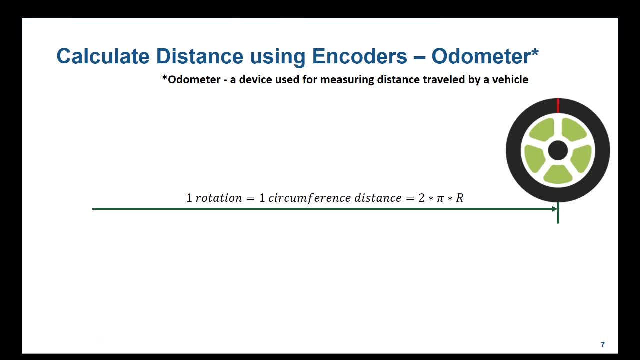 degrees, the wheel center would have traveled a distance equal to the circumference of the wheel. this circumference is given by the formula two times pi times R, where R is the radius of the wheel. knowing this, we can see that equals the number of rotations times the circumference. we can then substitute the: 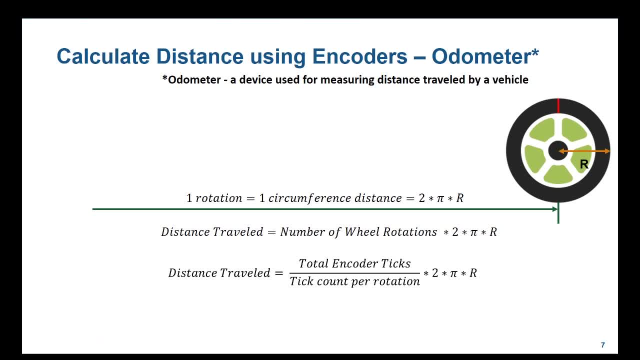 number of wheel rotations by the equation in the previous slide, where we compute wheel rotations using encoder ticks. it is important note that the tick count per rotation and the circumference are fixed values for most robots and need to be determined only once. this is because the tick count per rotation for 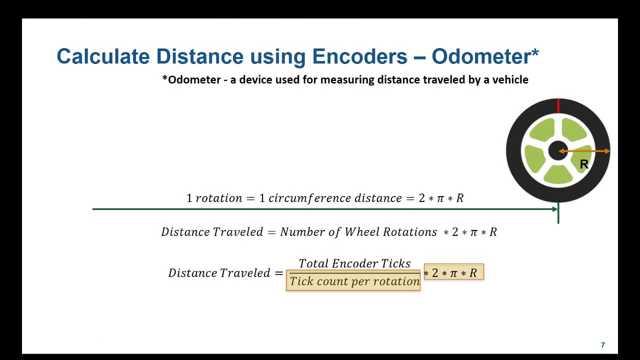 any given encoder sensor is constant. as noted in the manufacturer data sheet, the circumference depends on the radius of the robot wheel. this is also going to remain constant. the only variable is the total number of encoder ticks. we can think of this quantity as the input to our system. the output of the system is: 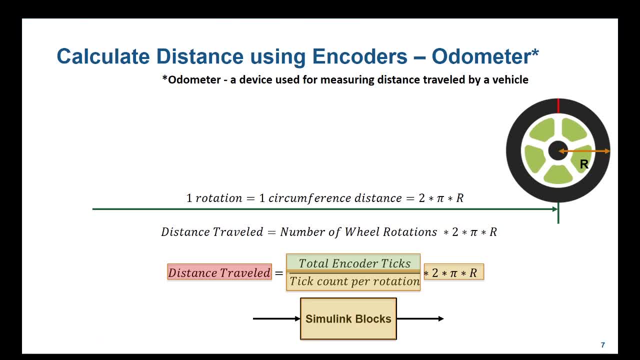 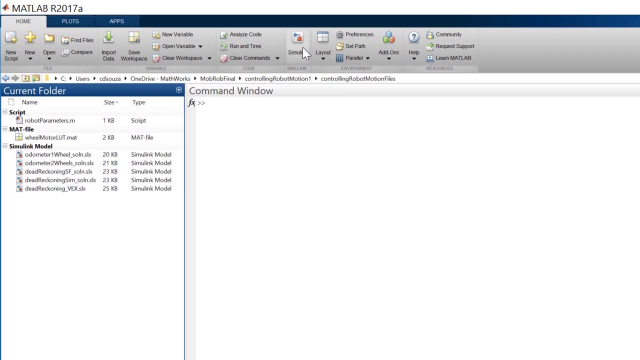 the distance traveled. let's see how we can implement an odometer in simulink. the input to our system is the distance traveled and the output to our system is the distance traveled. to this system are the encoder ticks and the output is the distance traveled. let's switch to MATLAB. to get started with simulink, select the simulink icon. 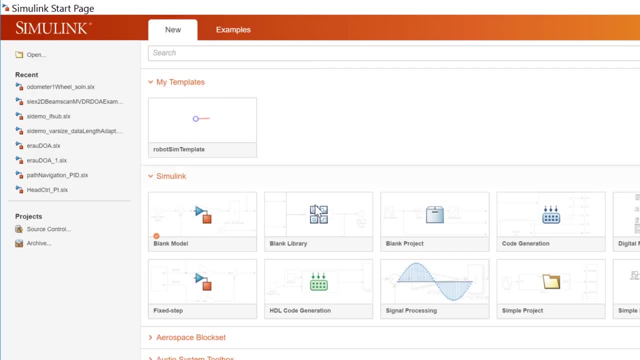 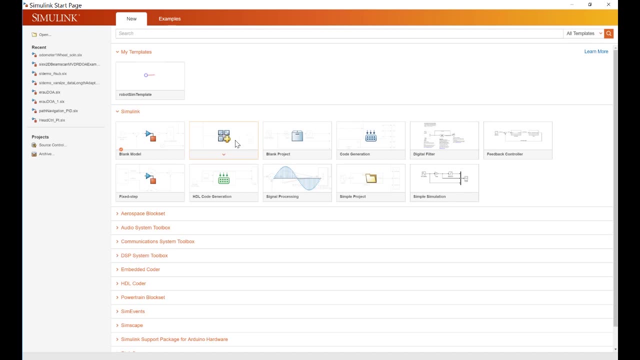 in the home tab of the MATLAB tool strip. this will open the simulink start page. the simulink start page contains a set of model templates which are useful for different applications. it also provides access to product examples, recently opened files and templates that you have previously created. 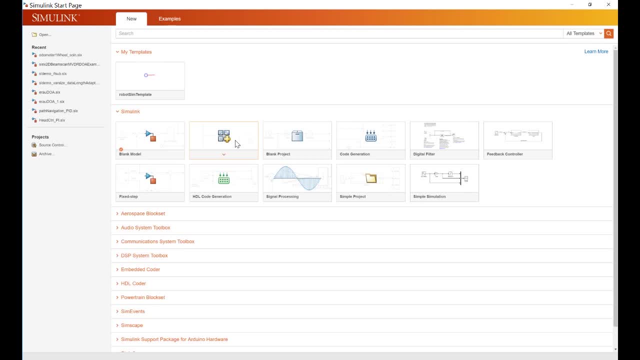 clicking a template will create a new simulink model based on that template. the simulink model window is where you visualize and simulate a block diagram of your system. to create a new model, select the blank model template over here to add blocks to this blank model. let's open the simulink library browser. 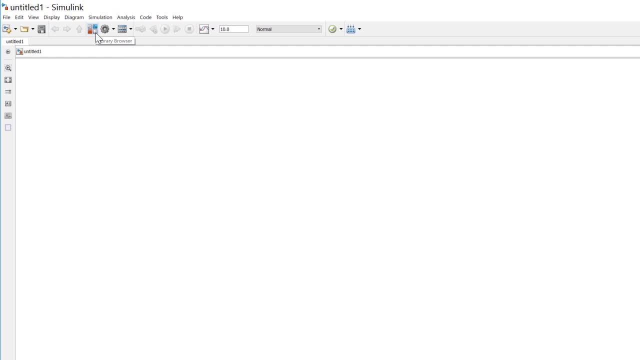 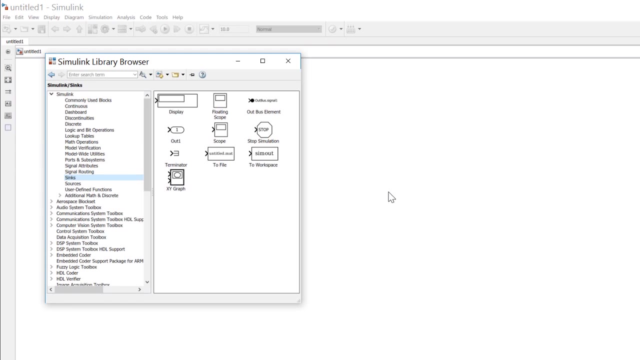 by selecting the library browser icon on the tool strip. the simulink library browser displays libraries in a list on the left hand side. to see the blocks contained in the library, select the library name. the blocks inside the library are listed in the right column. to add a copy of the library block to a 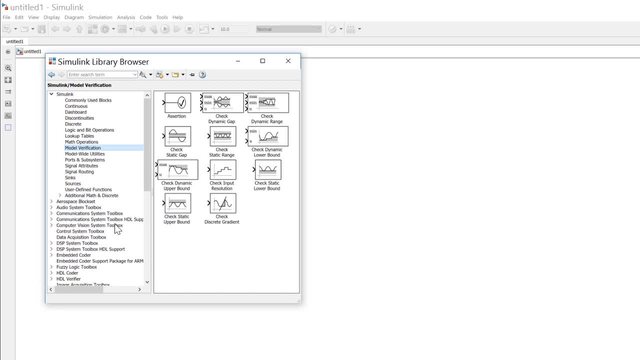 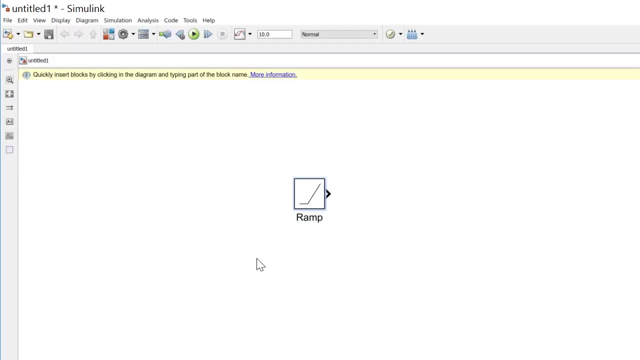 model. drag the block from the library browser to the block diagram. in order to build our first model, let's copy the following blocks: let's go into the sources library and choose the RAM block. let's click and drag this into the model. we will use this block to simulate an encoder sensor, a ramp means. 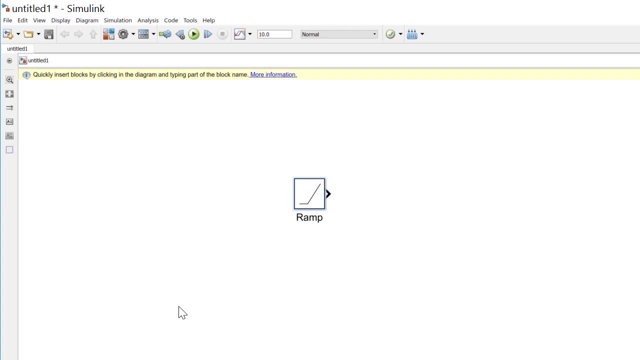 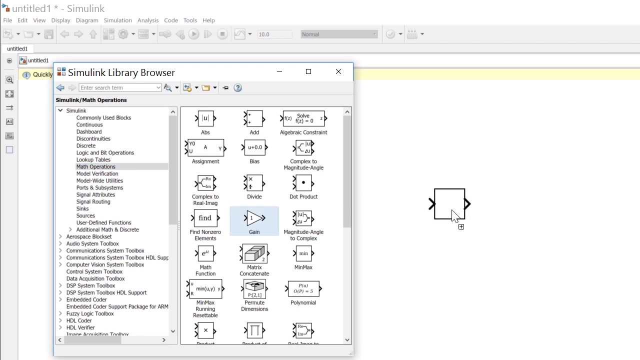 the signal rises with a constant slope. this is representative of an encoder behavior when the robot is moving in a straight line. the next block that we need to add is the gain block. so let's go back to the library browser and, under the math operations library, let's choose the gain block. drag and drop this in the 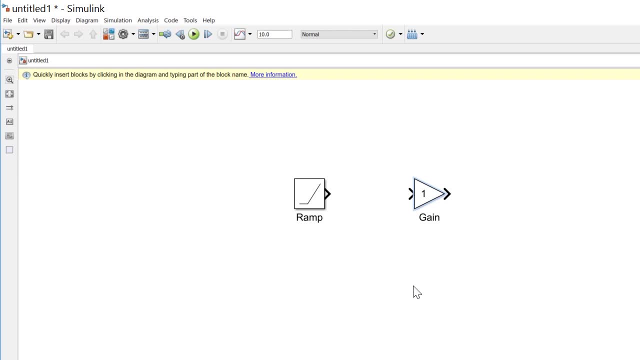 model. this gain block is used to convert the encoder ticks into distance traveled. since the output distance traveled is a constant multiplication factor of the input encoder ticks value, we use a gain block. and finally, we need to visualize the output of the system. so let's choose a scope block from the syncs library. it's going back to the library browser. 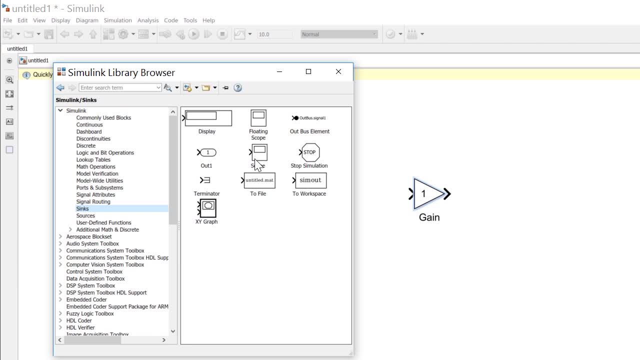 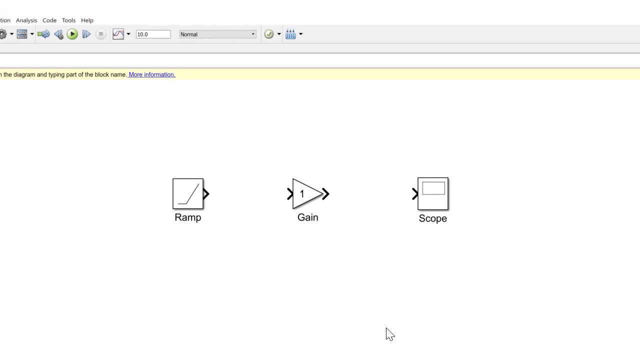 and under the syncs library, let's choose a scope block and add it to our model. now we just have these blocks, how are they going to interact with each other? we need to connect them. the output of the RAM block should be the input to the gain block to connect these. 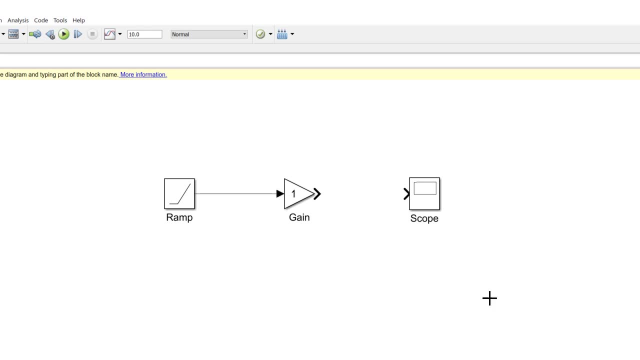 two blocks. left-click on the output port and drag it to its destination, and let's do the same for the gain block and connect it to the scope. next, it's usually a good idea to rename block in signal names to enhance the readability of the model. to rename the block, click the block label and edit it. let's rename the. 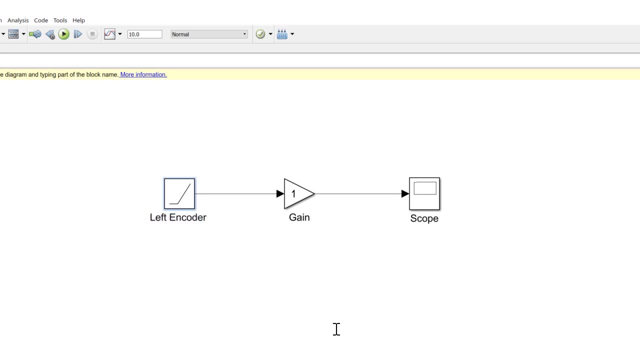 ramp to left encoder count. This signifies that it represents the left wheel ticks. Let's rename the gain block to ticks to distance and the scope block distance traveled. Let's also rename the signal that is the output of the gain block to left wheel travel. To name a signal, click on the signal and type in. 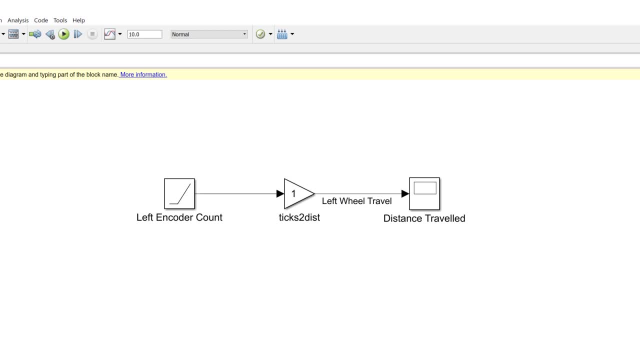 the name Recall that we have just dragged and dropped these blocks, connected them and labeled them. Next we need to define their parameters to make them describe our system or equations. We will leave the RAM to be at its default values. For the gain block, we will specify the equation that we delivered. 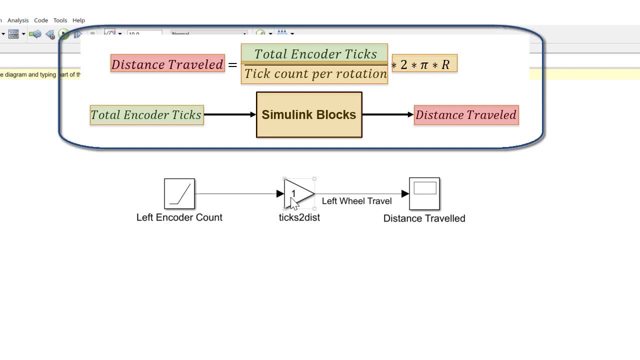 in the presentation. So let's double click on the gain block to open the block parameter dialog And let's specify the parameter values as 2 times pi, times wheel R divided by ticks per rotation. Note that the wheel R and ticks per rotation are variables. 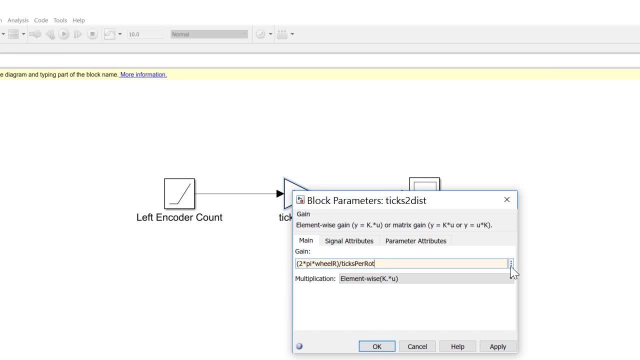 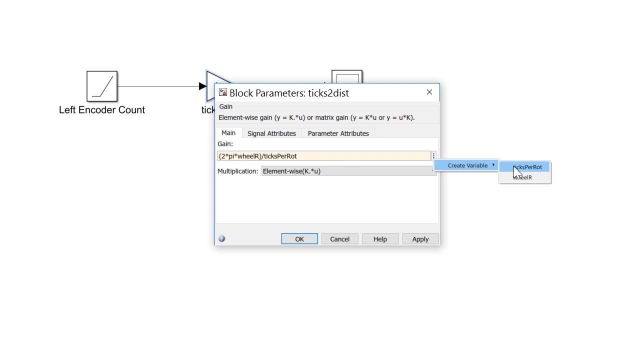 and need to be assigned. To do this, let's click on the ellipsis besides the dialog and choose the create variable option, and let's select ticks per rotation, Set the expression to the value. In our case, let's set this to an example value of 360, just like I'm doing. 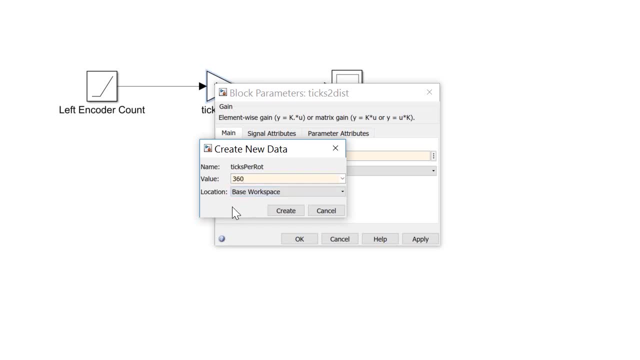 here. This means that it's 360 ticks for one rotation. Let's hit create and let's hit OK. Let's repeat the process for wheel R and set this value to be 0.052.. Now let's hit apply and let's switch back to the MATLAB window for a second. 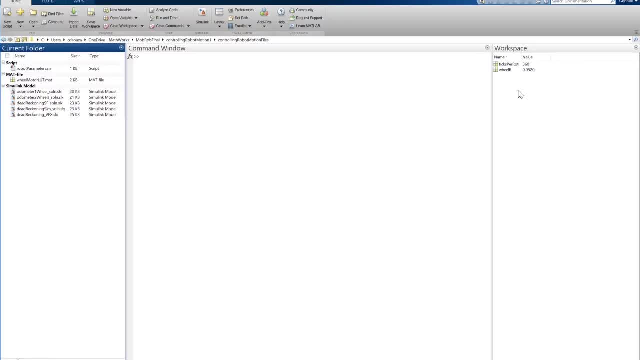 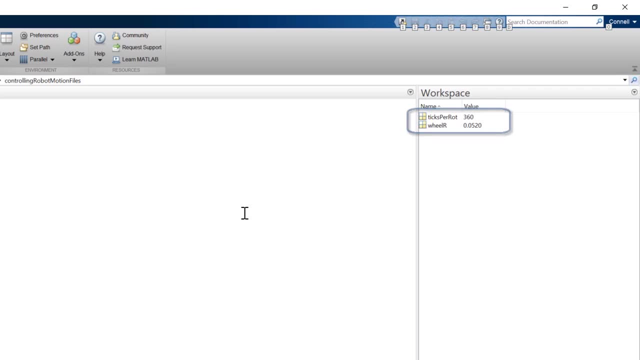 to see that these variables have been created in the command prompt. As you can see, ticks per rotation has been set to 360 and wheel R has been sent to 0.052.. Let's go back to Simulink. We can resize the gain block to see the equation. 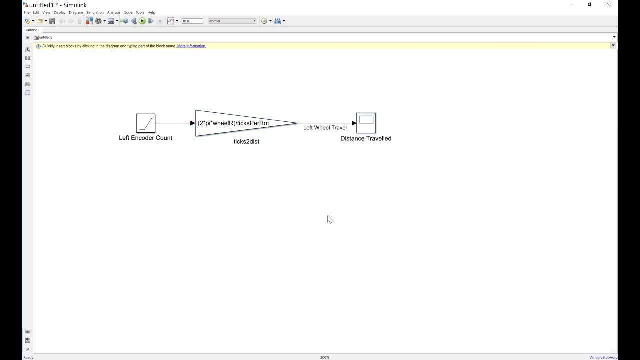 created here. just like I'm doing right now, Let's also visualize the input signal. So let's create a copy of the scope block. To create a copy, right click on the block and drag it. Let's rename this block to be encoder ticks. and now. 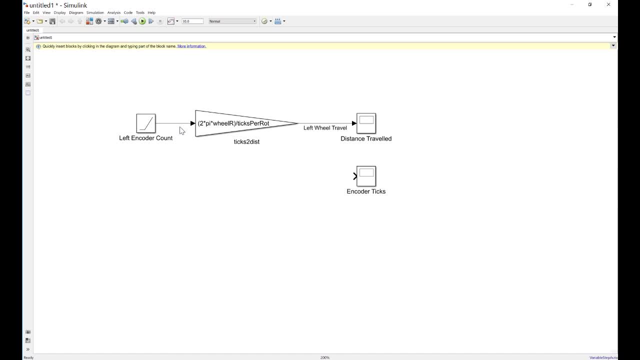 let's connect this to the output of the RAM block. To connect the signal, right click on the signal and drag. Now let's run our model and run your model by clicking on the green run button on the tool strip. Let's open the encoder ticks. 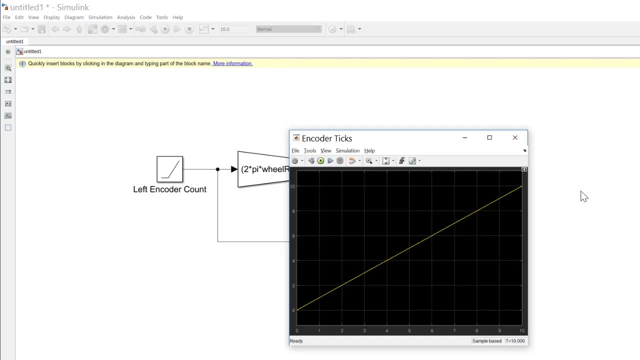 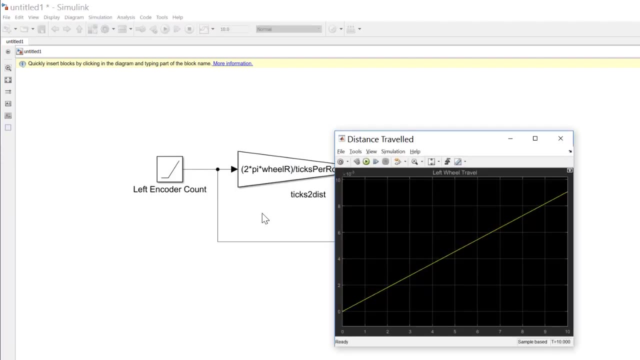 scope block. We see that the encoder has 10 ticks. Now let's go and open the distance travel scope. The distance traveled is close to 10, raised to negative 2 meters. The way the RAM block is set up, it outputs one tick per second, So let's run. 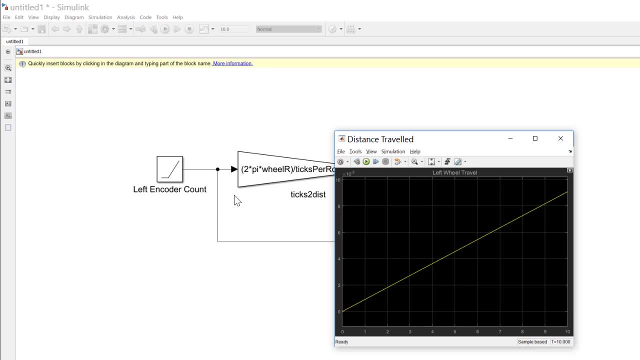 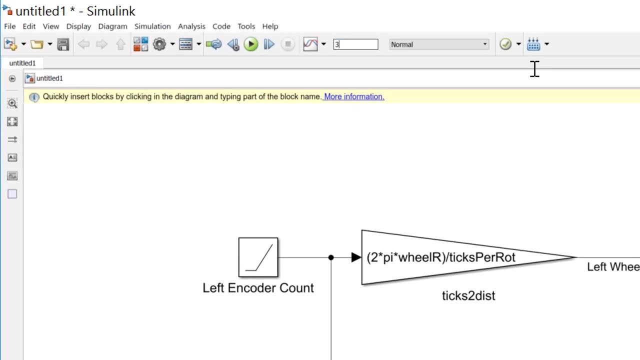 this simulation for 360 seconds. Let's go back into the model and let's change the simulation time up here Now, since our RAM block outputs one tick per second, if we run our simulation for 360 seconds, we expect our encoder to reach 360 ticks, which is equal to one wheel rotation. 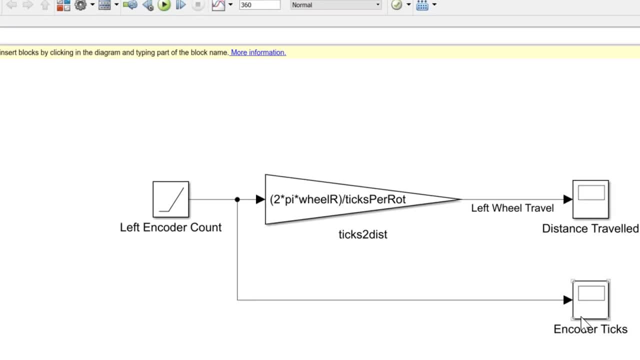 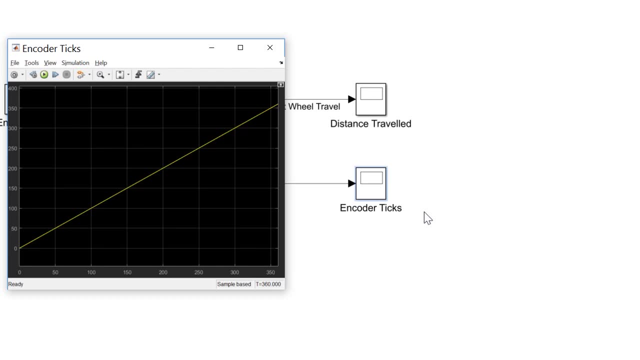 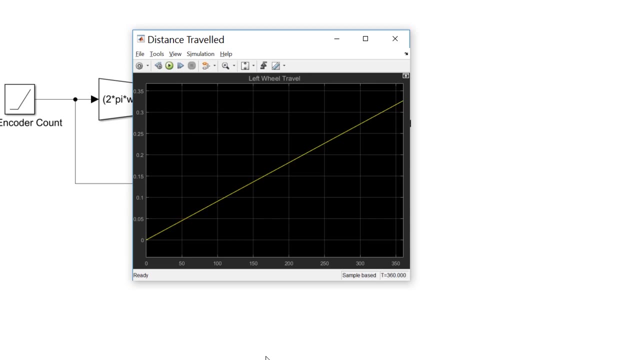 Let's run this model again. and now let's view the encoder ticks scope. We now see that the encoder ticks has reached 360.. Let's go back to the distance travel scope. We see that the distance traveled is about 0.325 meters. 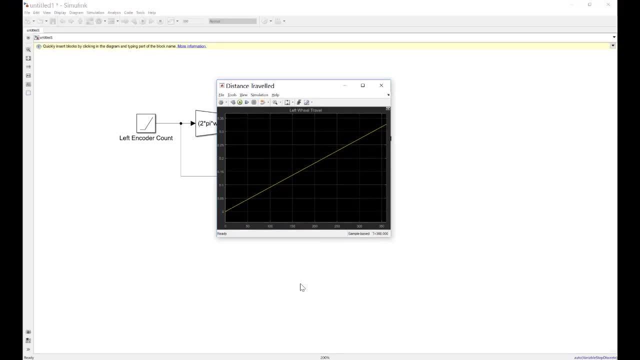 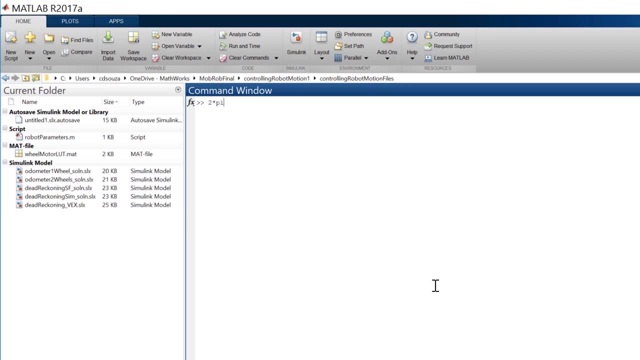 Let's compute our circumference in the MATLAB command prompt. Switch back to MATLAB. We know that our circumference is equal to 2 times pi times the wheel radius, which is 0.052.. We see that these results match. Let's look at the big picture. We can now. 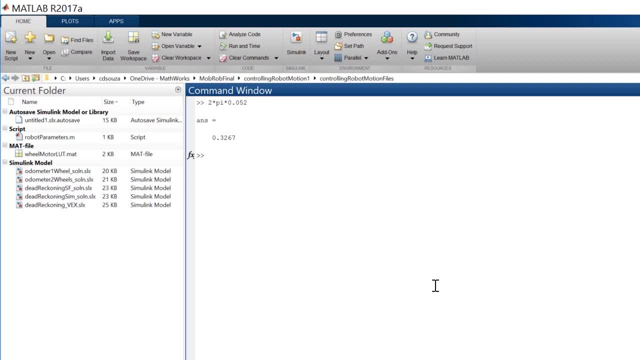 use this simulation to calculate the distance traveled for a given number of ticks or, back calculate the number of ticks required to move a distance. The next question would be: this is for the left wheel alone. What about the right wheel? What about the robot as a whole? Let's go back to 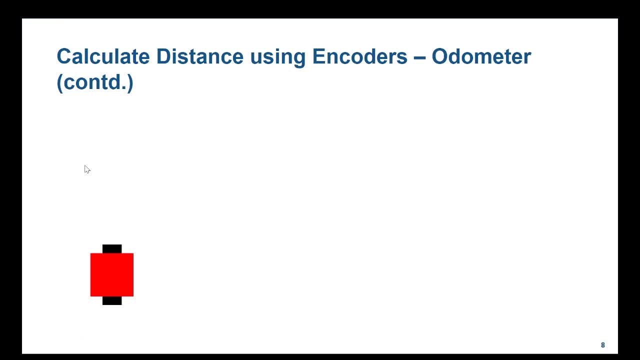 the presentation and look at this. Here is an example robot. We are looking at the top view of the robot. So the red block is the robot body and the black blocks are the wheels. Suppose the start and end points are here. Now, when your robot moves from the start to end like this, the distance 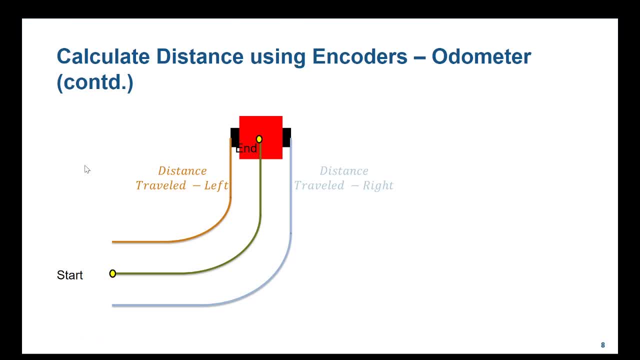 traveled by the right wheels and the left wheels are different, as shown here. However, we are interested in the distance traveled by the right wheels and the left wheels, So let's go back to our model and get the average of the distance traveled by the center of the robot, which is 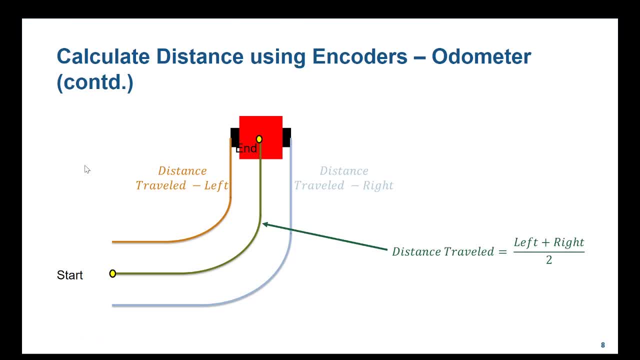 denoted by the green line. This is easily obtained by taking the average of the left and right distance traveled. We have already implemented the distance traveled equation for the left wheel. Let's reuse this for the right wheel and complete the calculation by taking the average. Let's go. 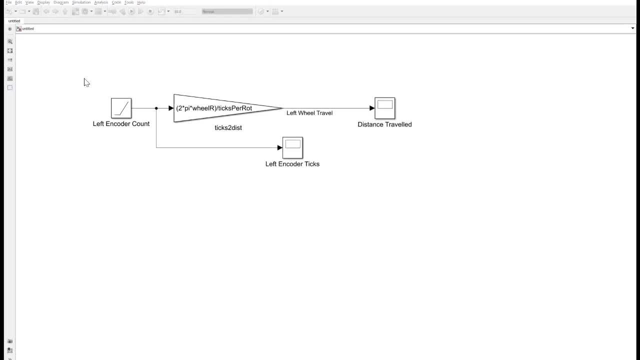 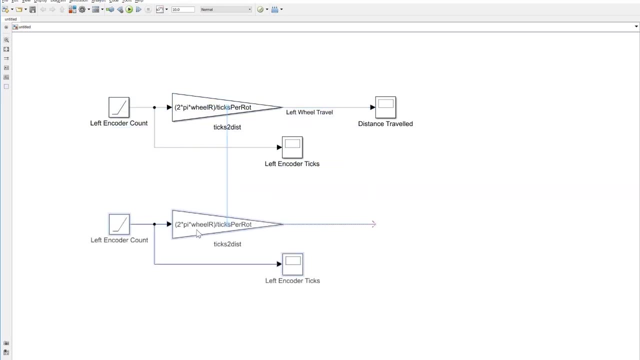 back to our model. Let's copy the left wheel blocks. You can copy a group of blocks by selecting the blocks that need to be copied, right-clicking and dragging, just like we did earlier. Now let's rename these blocks to be the right wheel blocks. So the RAM block would be the right encoder count. 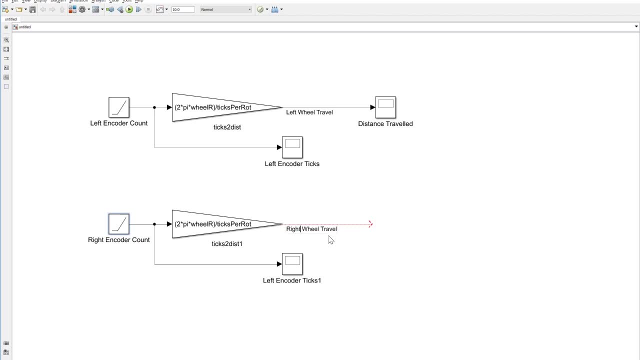 the output signal of the gain block would be the right wheel travel and the scope would be right encoder tricks. Now we need to take an average. In order to take the average, we need to first add the two quantities and then divide them by two. So let's go back to the Simulink library browser and from: 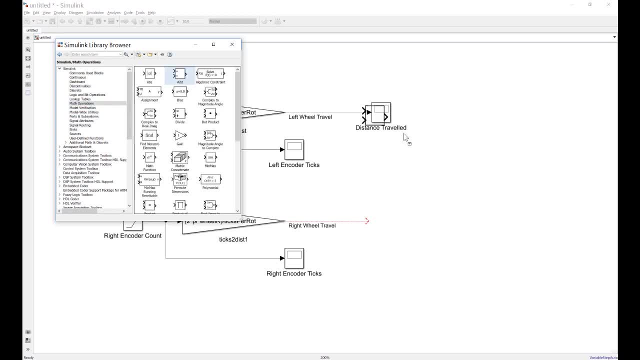 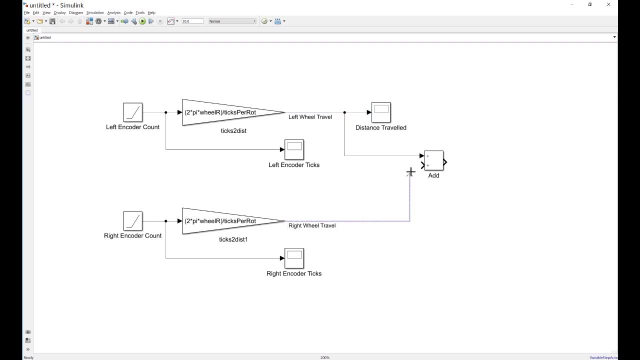 the math operations library. let's choose the add block and drag it into our model. Now let's connect the left wheel travel and the right wheel travel to the add block. Let's delete off this portion of the signal for a quick second here. 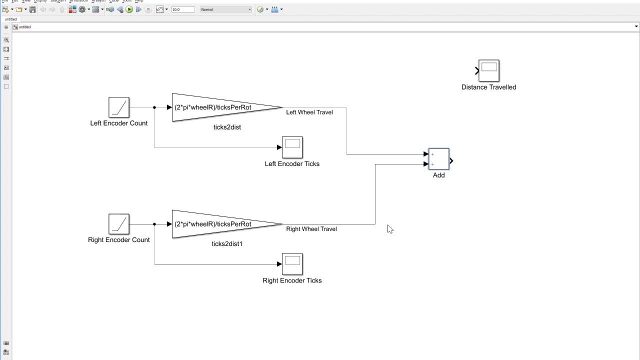 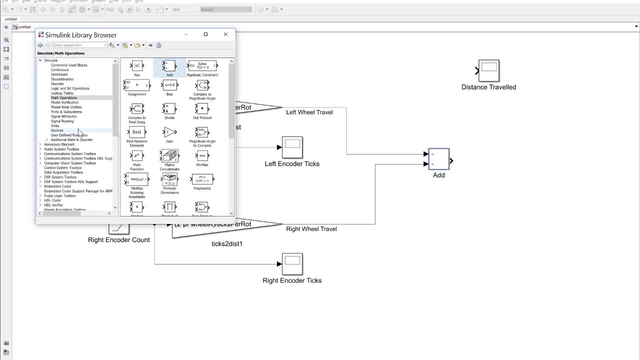 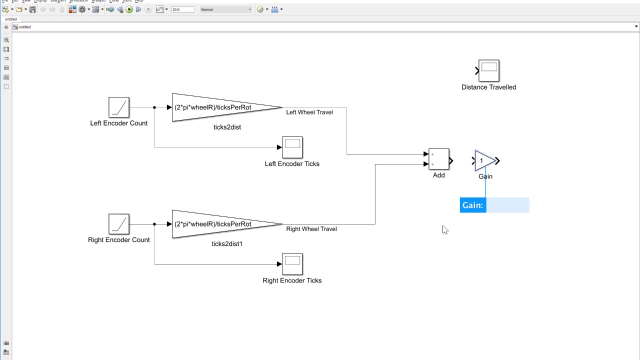 Now, after adding the two quantities, we need to divide it by two. Dividing something by two is the same as multiplying it by 0.5.. So let's add a gain block from the Simulink library browser and set the gain parameter to be 0.5.. Another easy way to set the gain parameter is by entering: 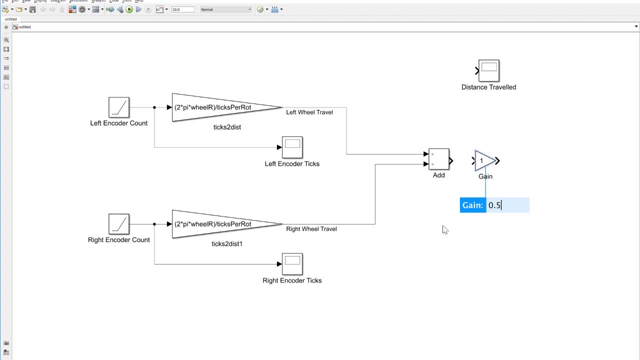 it into the banner that pops up when you insert the block into the model. Now let's connect the add block to the gain block and the output of the gain block to the distance traveled scope. Now let's test for the scenario where the robot is rotating. 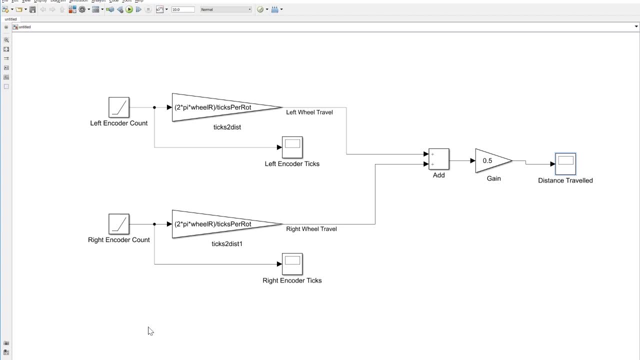 in one place, That is, the left wheel is rotating in the forward direction and the right wheel is rotating in reverse at the same speed. So let's set the ramp input slope for the right wheel to be negative one. Let's open up the right encoder, count ramp block and set the slope to be negative. 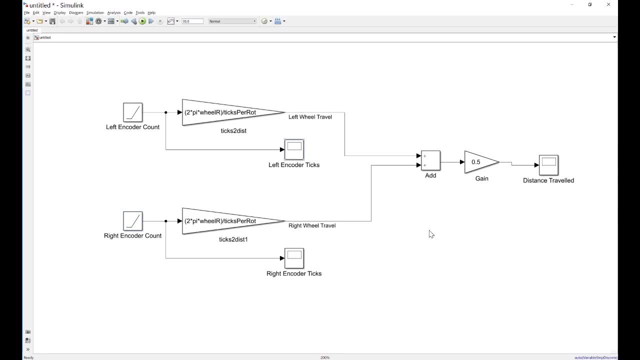 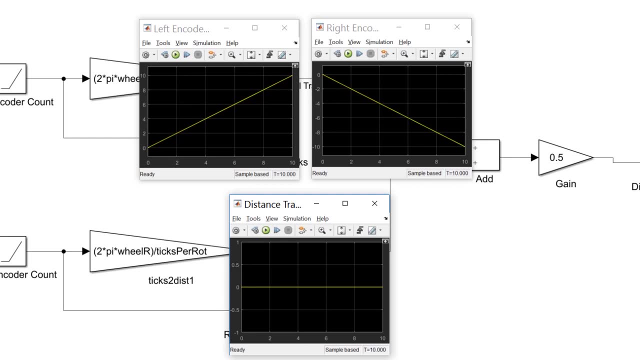 one. Now let's run the model. Let's open up all the scopes. We see that the left and right encoder scopes are non-zero values. That means the wheels are rotating. However, the distance traveled is zero because the robot has technically not moved anywhere else. 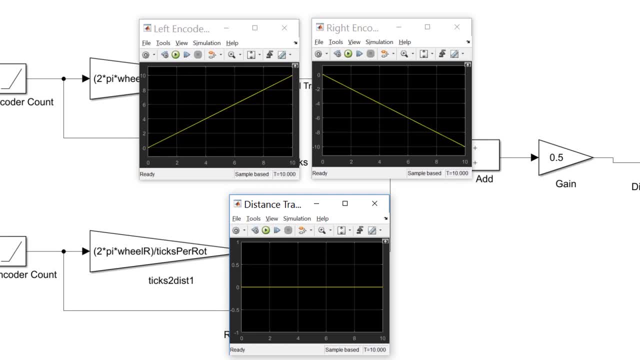 It has just been rotating in one place. We can use this model to do tests from actual sensor data to figure out how far the robot has moved. So, given the left and right encoder values, we have successfully computed the distance traveled. Let's go back to the presentation. 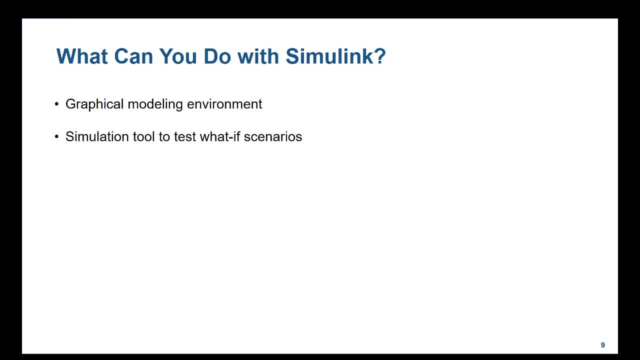 for a recap, We just built our first Simulink model. We can use the simulation environment to build an odometer from encoder sensor inputs. We see that Simulink can be used to generate example inputs and look at outputs. In addition to this, it can also be used to implement mathematical equations. 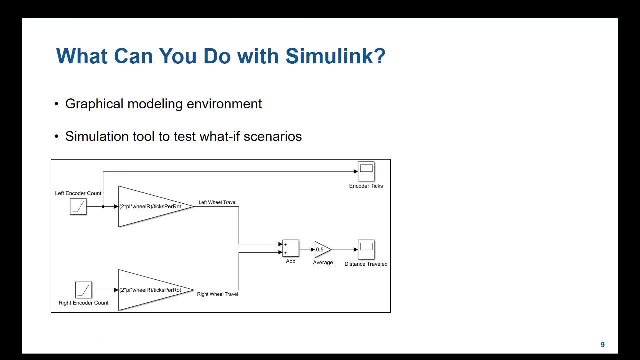 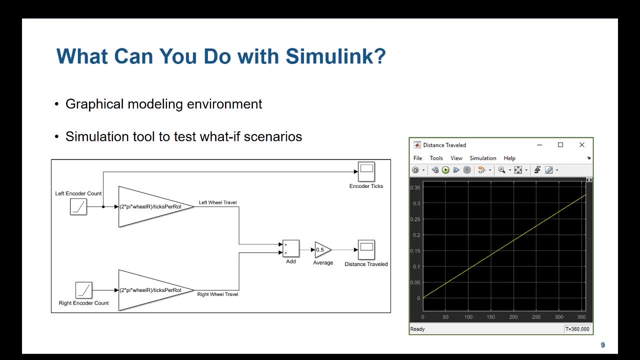 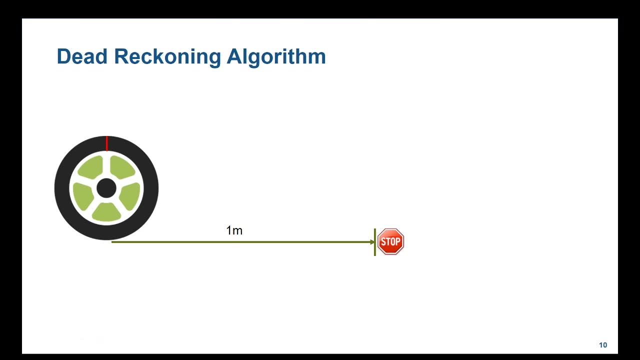 The simulation environment helps in testing what-if scenarios. For example, using our model, we can check how far the robot has moved given an encoder input. The next step is to implement the actual algorithm. So far, we have been implementing math. What about logic? Many of the robotics algorithms involve logic and mode-based operations. 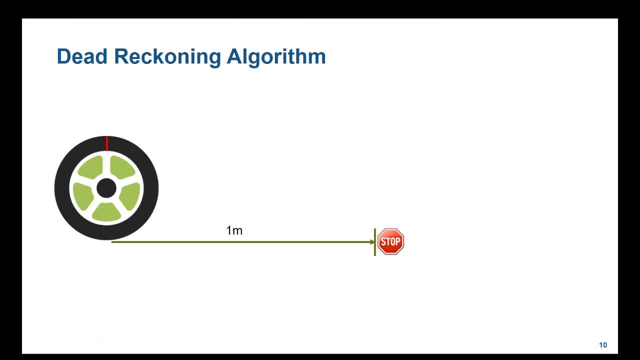 Let's take a simple example Based on the model we just built. what if we want to monitor the distance traveled and then stop the robot once we have reached 1 meter? If we visualize this in a flowchart, we also have somewhat of a radiator of time and water. 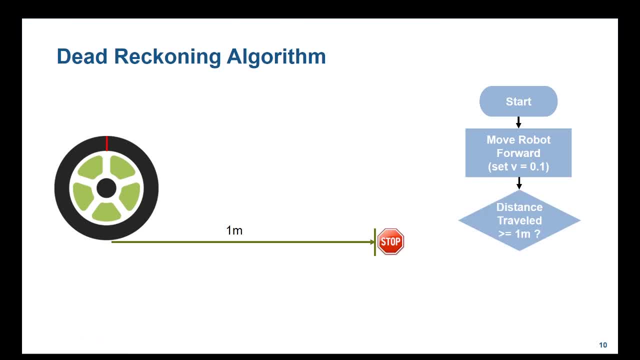 So we can actually do this. It looks like the robot is moving as if it's speeding. Let's check if the data from the robot can be resurrected in 1 meter. This gives us the starting point for testing our algorithm. So first we begin execution of the algorithm, then we will have the robot move forward. 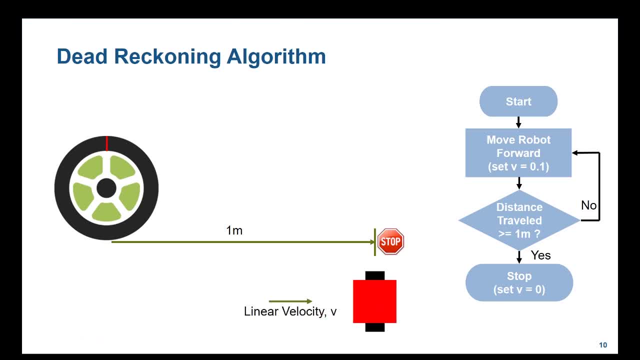 Next we check if the distance travelled is greater than or equal to 1 meter line and Omega, which is the angular velocity and that represents how fast the robot is rotating in one place. So to move the robot in a straight line, we set V equal to a nonzero value, and to stop, we set it to zero. Omega remains zero for. 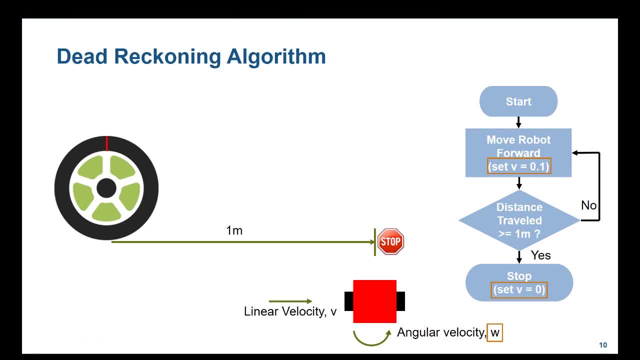 straight line movements. since we are not rotating the robot, Let's go back to Simulink and see how we can implement the flow chart logic to move the robot for one meter. In the model that we are working on, we will use state flow charts. 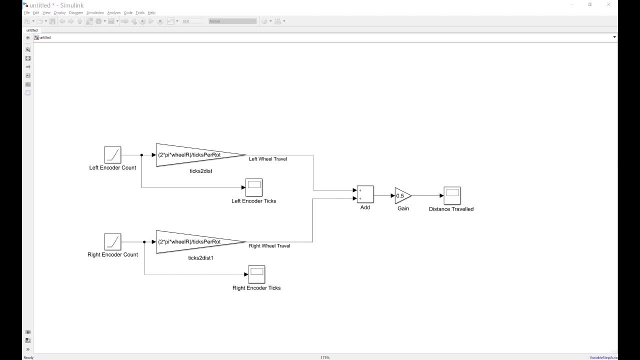 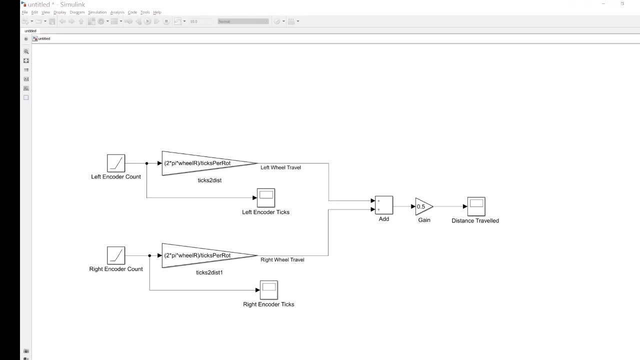 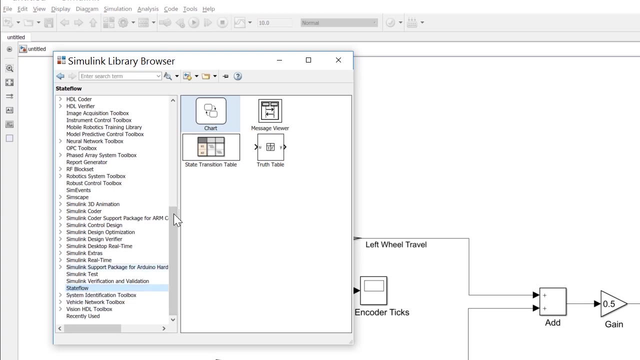 to build the logical part of our algorithm. State flow is great at modeling modes of operations and making logical decisions. To add a new chart to a model, let's open the Simulink library browser and scroll down to the state flow library, and from the state flow library let's drag the chart. 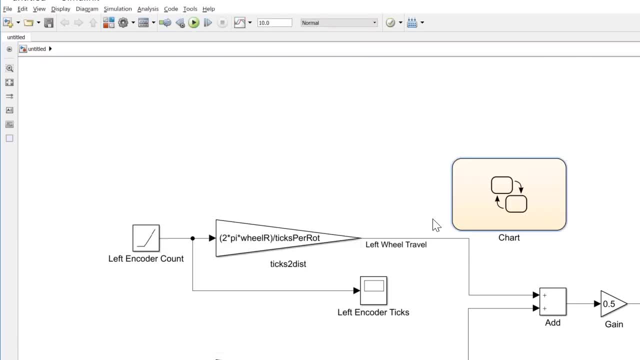 option into the model. This chart should take in the computed distance traveled as input and then output a velocity value. Let's double click on the chart block to open up the state flow chart. Recall that we have two modes of operation in our algorithm: a move forward mode and a stop mode To model. 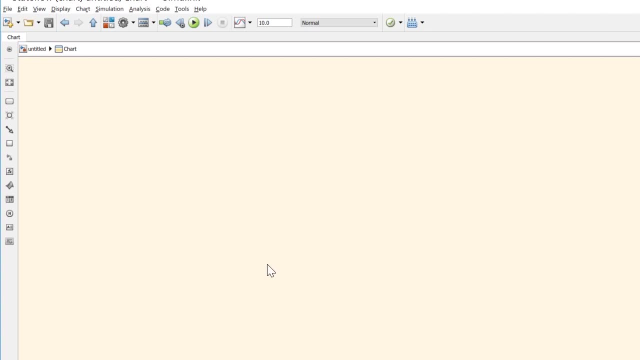 this. we will use states. To add a state to the chart. select the state option on the toolbar on the left and drag it to the chart. Drag it into the model. The first state of the chart is the default state. This is denoted by the default transition here, which is where the program execution. 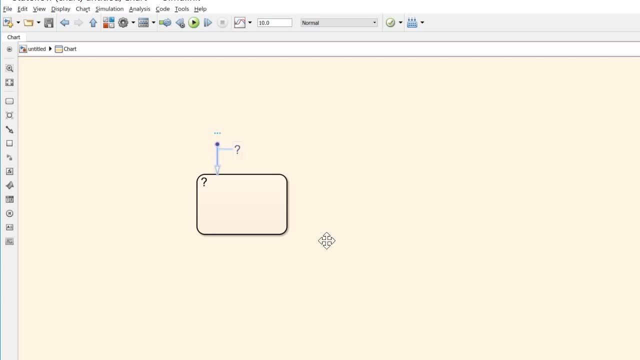 begins. We can add a comment here by double clicking on the transition and editing the question mark To add a comment. add the percent sign and then type out your comment. Let's call this the start To add the second state. let's make a copy of the first state. 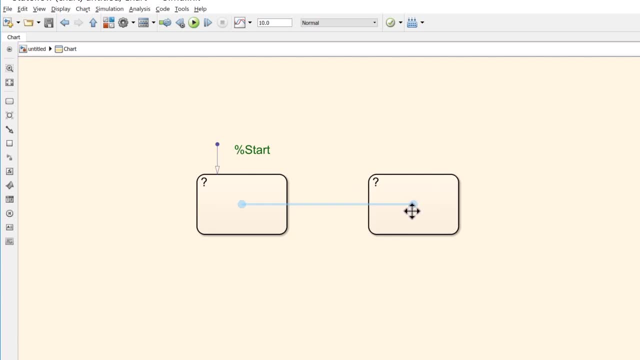 Copies of states can be made in the same way like we make copies of blocks in Simulink. Now we have two states. We must label each state with a valid name. Valid names are any alphanumeric or underscore characters without spaces and don't start with the number. Look at the link in the resource section to get a full. 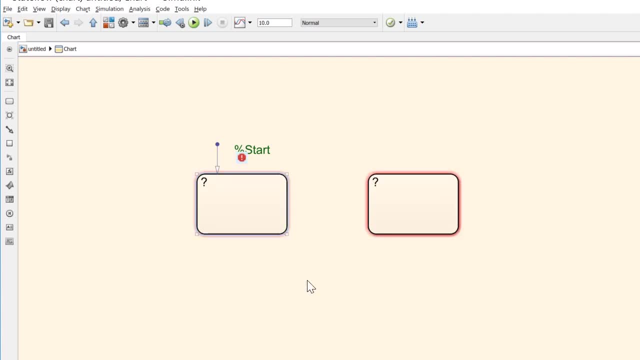 list of rules for naming the state. Let's name the first state as the move forward state and the second as a stop state. Now we need to define the state execution statements. What should these states be doing? They need to be controlling the velocity v Move forward. 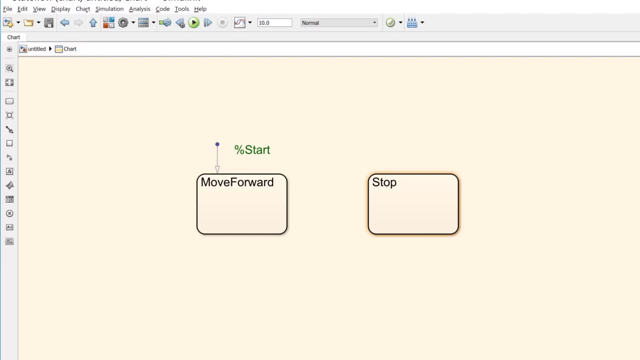 should set the v to 0.1 and stop should set the v to 0. So let's type in: v equals to 0.1 in the move forward state. Now we see that state flow automatically adds another word, namely entry to the. 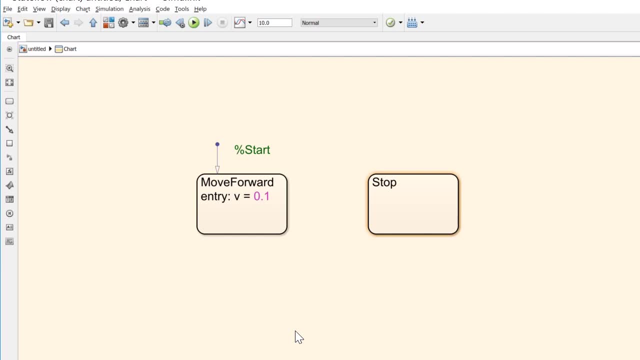 description. This means that state flow will execute the statement once when it enters the state. We can see this better when we run the model. For now, let's also set the velocity in the stop state to 0. So v equals 0. And, as you can see, the entry. 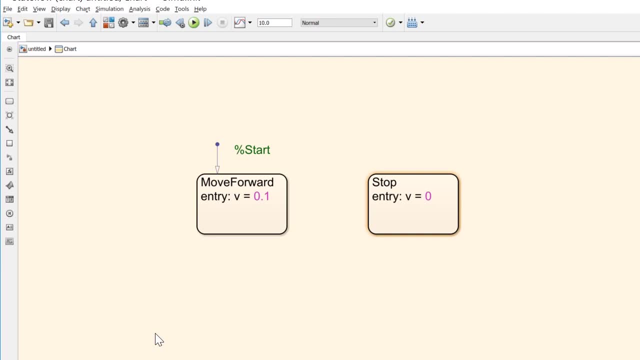 word has been added here as well. Next, we need to define the condition at which we will transition from the move forward state to the stop state. We already know this condition to be that the distance traveled has to be greater than or equal to 1 meter for this to happen. We know that our 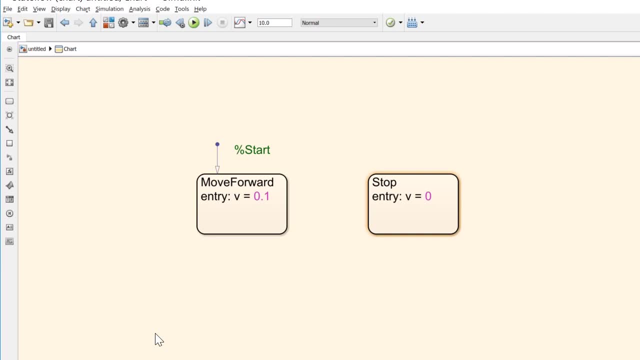 robot has to stop once it reaches the 1 meter mark and hence the transition condition will be that the distance traveled is greater than or equal to 1 meter. To define this, we will use transitions To create a transition. move your pointer to the edge of the move forward state until the crosshairs. 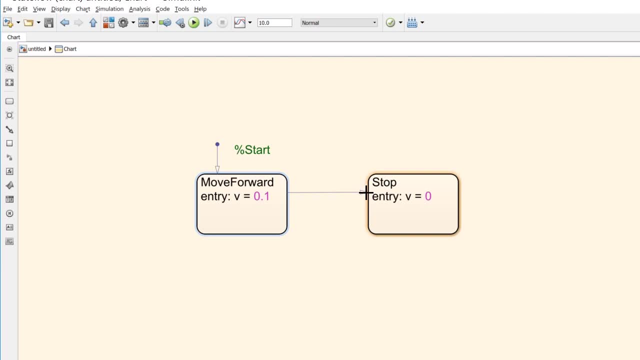 appear, and then click and drag until the destination, which in our case is the edge of the stop state, and then release the mouse button. We have now defined a transition path. Next, we need to define on what condition does this transition happen? So let's double click on the transition to see a. 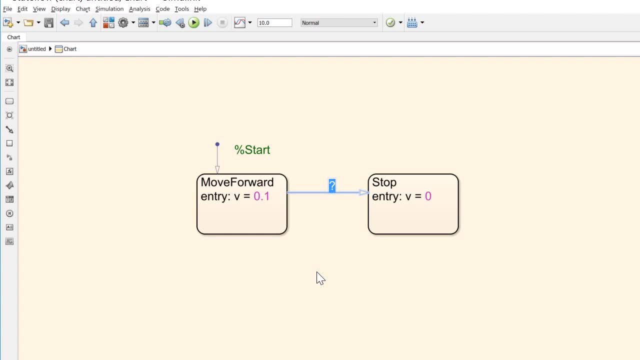 question mark pop up. Let's type in the condition that we discussed earlier, which in our case would be dist traveled is greater than or equal to 1.. Then click outside to see that state flow automatically adds square brackets around the condition. This is a necessary syntax. Most times, state flow 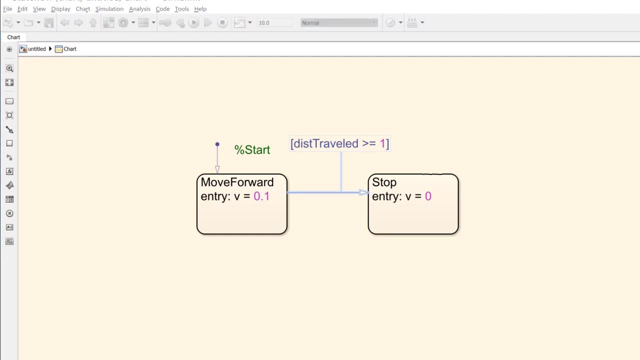 does this first automatically Other times. do note that the conditions need to be enclosed in square brackets. Now our algorithm is complete. Next, let's think about where the dist traveled value is coming from and where the V value is going to. These are input and output variables in our chart, and they 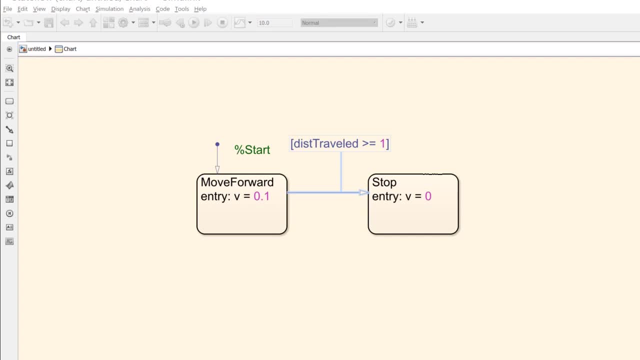 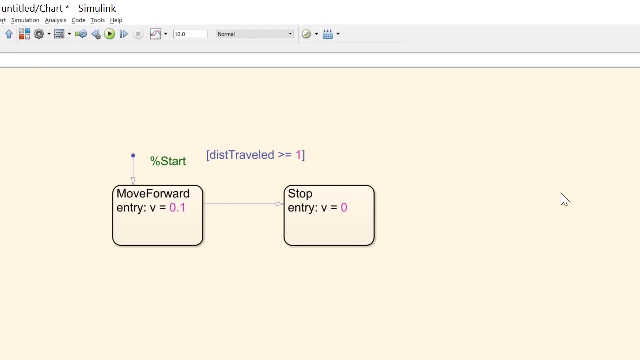 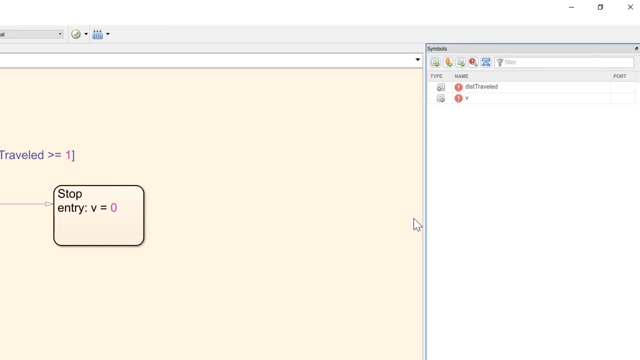 need to be defined as such. To do this, let's go to the view tab on the tool strip and select the symbols option. This pulls up a pane on the right hand side of the screen that has the symbols already over there. Here we can see that state flow already recognizes these as unresolved. 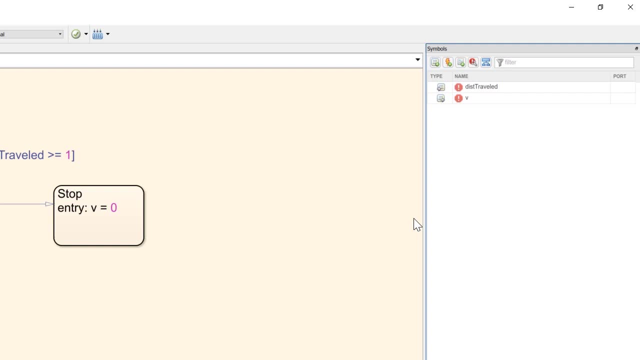 symbols. We can resolve these by clicking on the exclamation button on the top over here, just like I'm doing right now. Then we can verify if state flow has resolved them correctly. And, as we can see, dist traveled is an input and V is an output, which means the 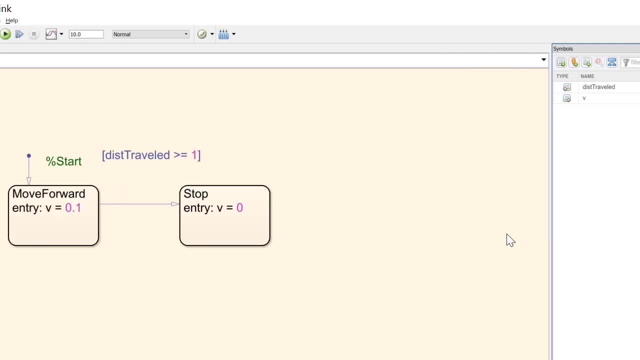 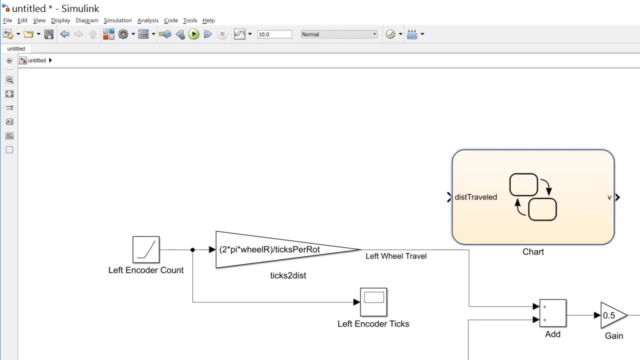 state flow is right. Let's go back up one level in the model through the breadcrumb over here. Now, when I resize the chart, you can see that an input and an output port has been created to the state flow chart and now looks like any other. 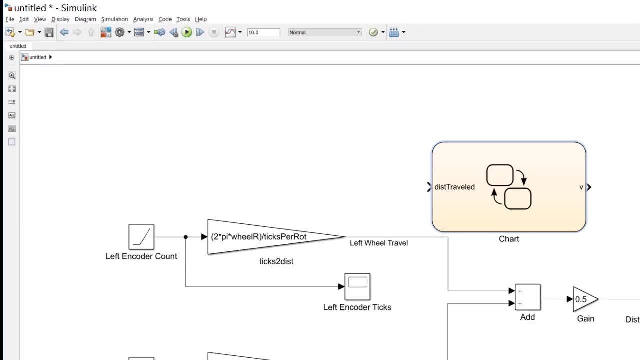 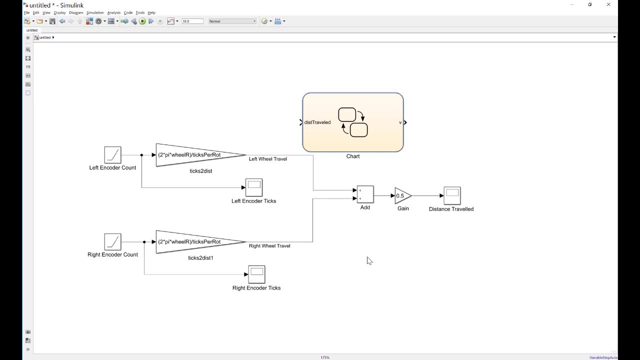 Simulink block which accepts inputs and outputs. Where does the dist traveled value come from, though? We've already calculated this and we can use it here as the input to the distance travel scope, So let's add the chart to our model. Again, recall: you can connect a signal by right clicking on. 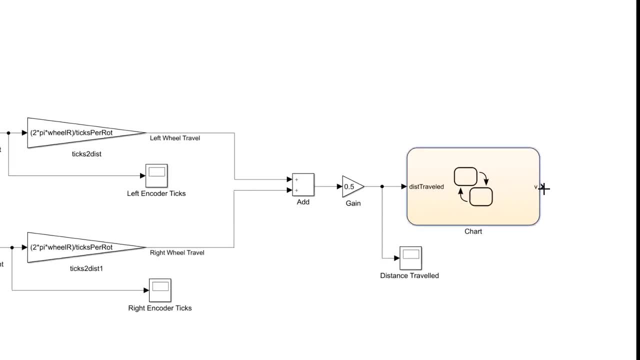 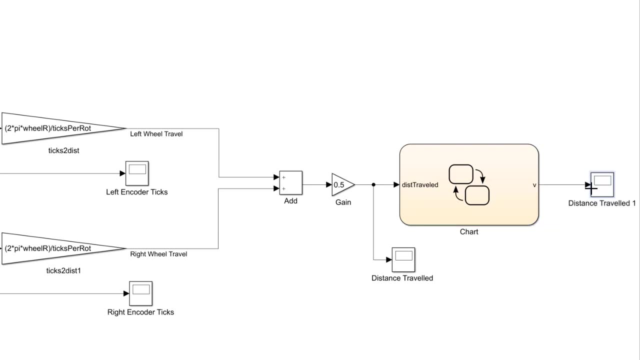 the signal and dragging it. Now let's connect the output of the chart V to another scope. So let's make a copy of the distance travel scope and connect the output V to it and let's rename this as velocity. Now remember to change the. 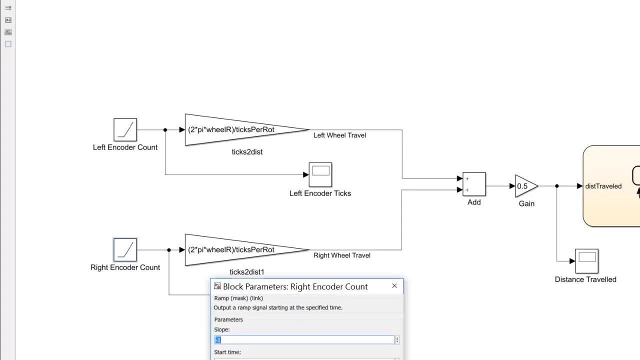 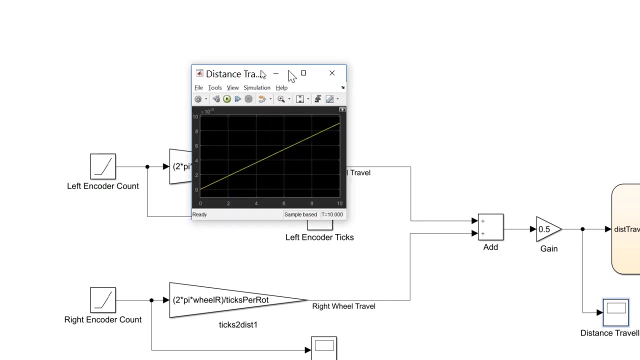 slope on the right encoder count ramp block To positive 1 to signify that our robot is moving in a straight line. Let's change the slope to 1 and hit enter. Now let's run the model and let's take a look at the distance travel scope. As you can see, this the value on our distance. 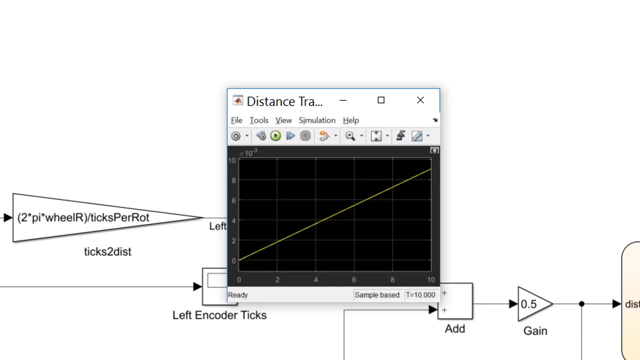 travel scope is a lot less than 1.. Recall that our algorithm is only doing something interesting when the distance travel becomes greater than 1.. So let's run the model for a long time So we can see what happens. So let's go back and change the simulation time on. 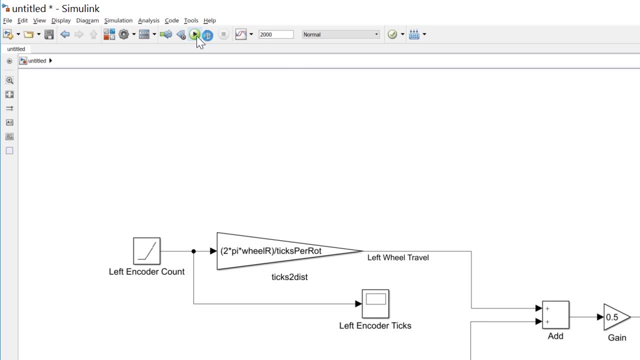 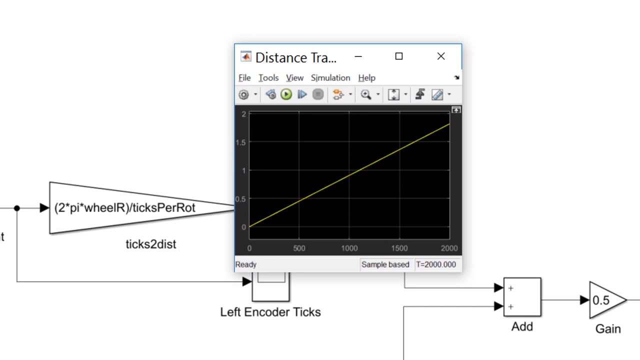 the top tool strip to 2000. and now let's run the model again. Now we can see that the distance traveled has gone beyond 1.. Let's approximately make a note of when it crosses 1, which looks to be around 1100.. Let's open the velocity scope Over. 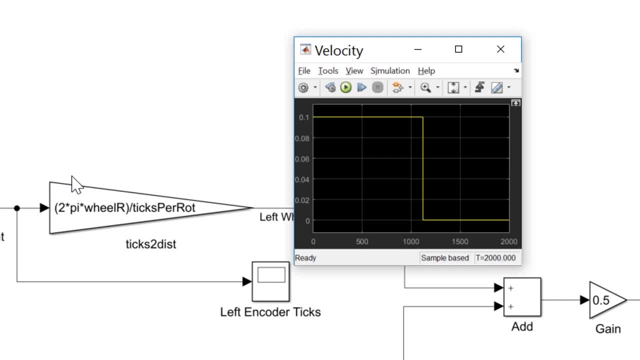 here we see that initially the velocity is 0.1 and then at around 1100, it jumps to 0. So our algorithm works. Let's go back inside the state flow chart and understand this a little more. Let's right-click on the distance. 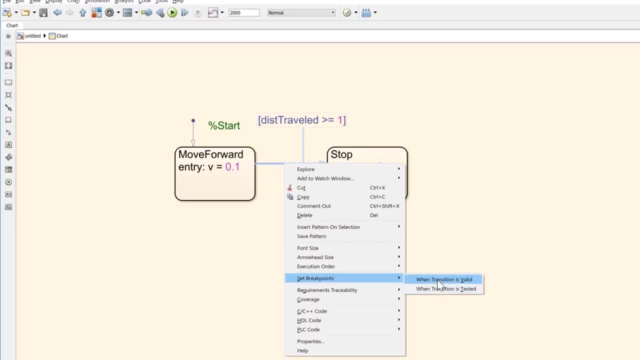 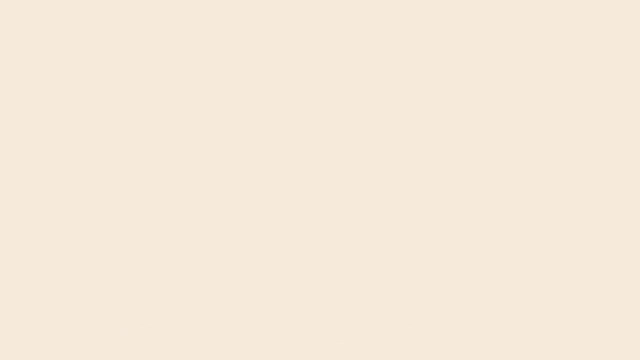 travel transition and set a breakpoint when the transition is valid, Just like I am doing on the screen right now. And now let's run the model again. We see that the execution has stopped in the model and it has stopped around 1120.. So we will correct the. 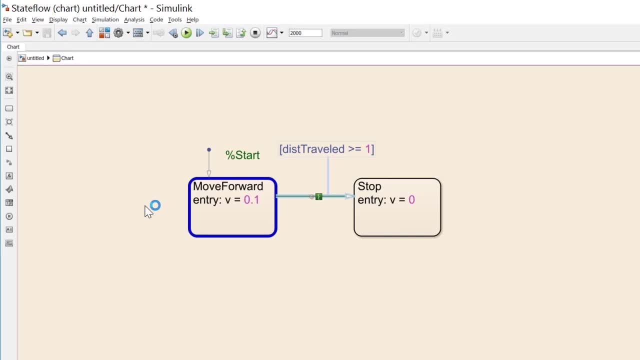 condition that this condition was true around 1100.. Now we can use the step mechanism here to see a step-by-step execution of our algorithm. So let's step through this. once We can see that it has now moved to the stop state. We can create breakpoints this way in various parts of our chart to help us. 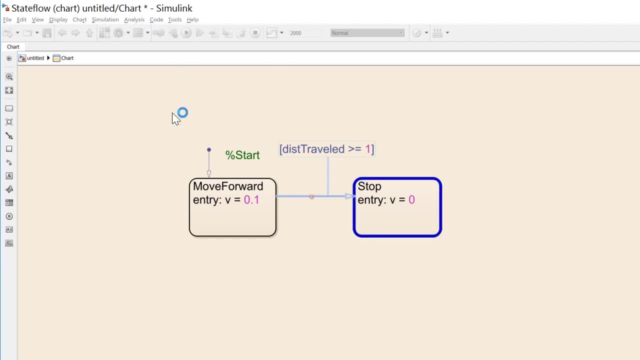 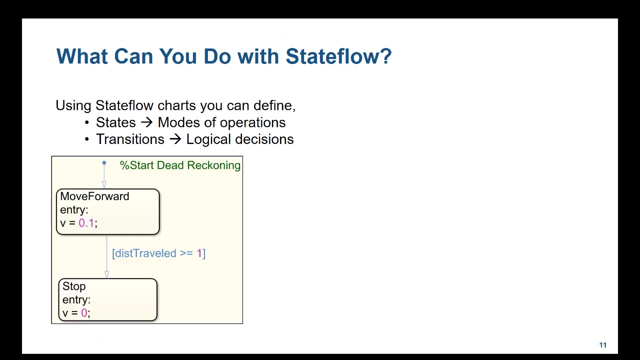 debug our algorithm. Let's hit the run button again to finish the execution. We have now successfully created a dead reckoning algorithm. Let's go back to the presentation and do a small recap. We just built our first state flow chart. We use states to describe the two modes of operation of our robot and we use transitions to 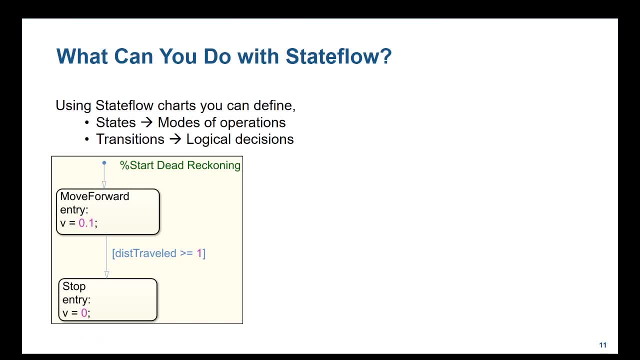 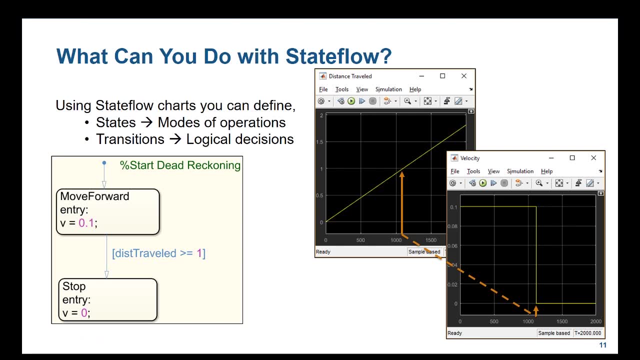 test for logical decisions in our algorithm. In our example, the moment our robot crossed the one meter mark, the velocity value went to zero. However, we can note here that our input sensor is just a simulated value. We can see that the velocity value of our robot is now 0.1.. We can 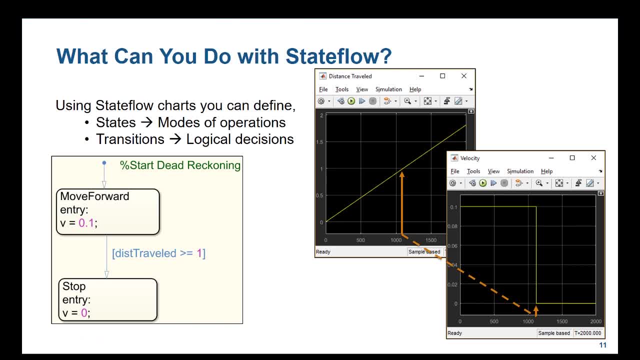 see that the velocity value of our robot is now 0.1.. This is an open loop system, which means that there is no connection established between our robot velocity and the input encoder value. We will be able to test for more scenarios if we have the input encoder value reflect our real system. 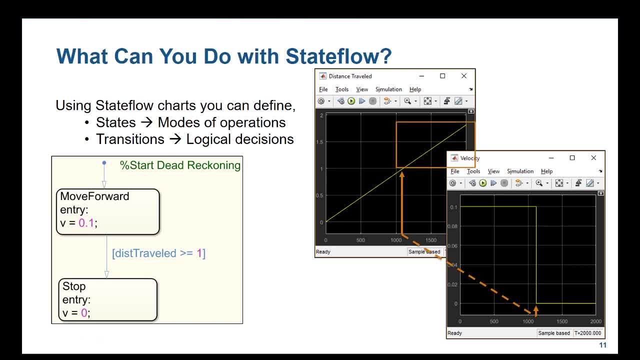 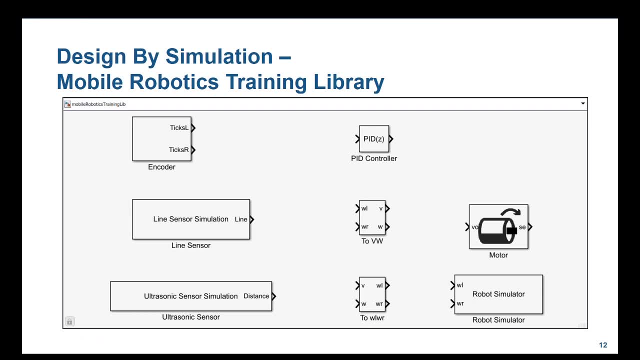 output, In other words the distance value, should stop increasing as soon as the robot velocity reaches zero. To do this, we will be using the mobile robotics training library to train our robot. This library, like any other Simulink library, has several blocks in it. It. 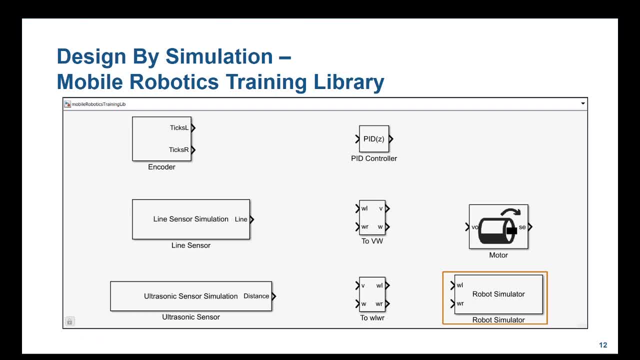 has a robot simulator that can help us visualize a robot given right or left wheel angular velocities. Note that these are wheel angular velocities, which are different from the V and omega values we discussed earlier. We also have a few utility blocks, For example to convert V and 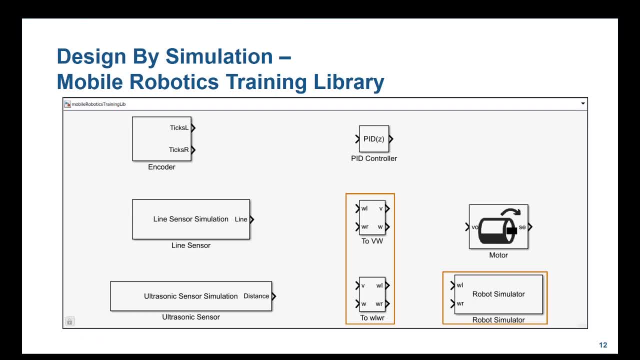 omega to omega L and omega R variables. We also have various sensor simulations that is tied to the simulator to give us the desired closed-loop tests, namely encoders, line sensors and ultrasonic sensors. We will take a look at these blocks in more detail next. So, coming back to the model that 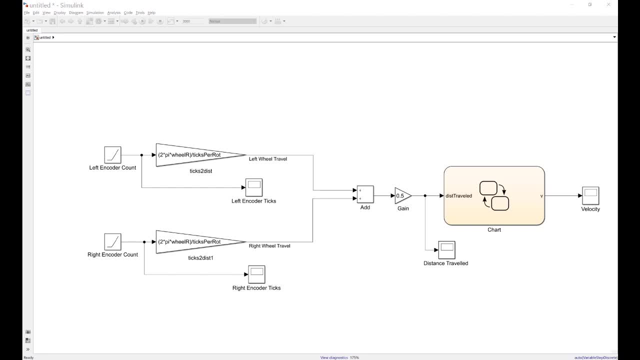 we were working with. now, instead of the RAM blocks, let's use the encoder blocks from the training library. So first let's delete the two RAM blocks And then let's open up our training library. So first let's delete the two RAM blocks And then let's open up our training library. So 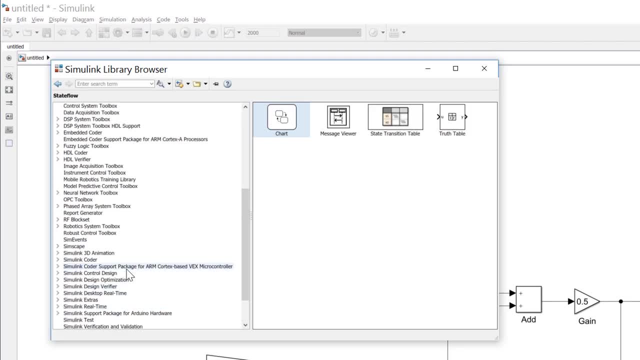 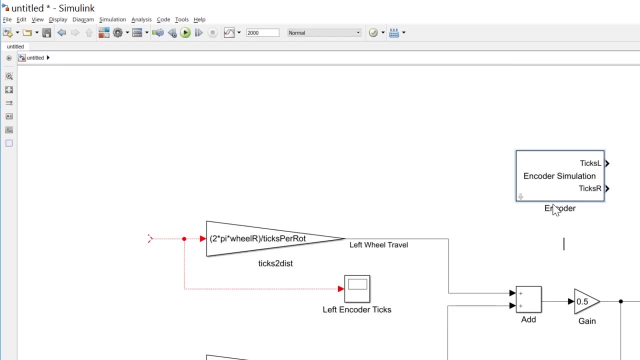 let's open the Simulink library browser And let's look for the mobile robotics training library, which is right here, And let's drag and drop the encoder block from the library into the model. Now let's connect the right and left outputs to the appropriate blocks in our model. 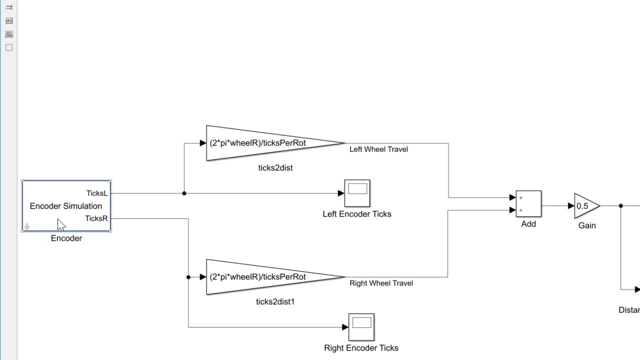 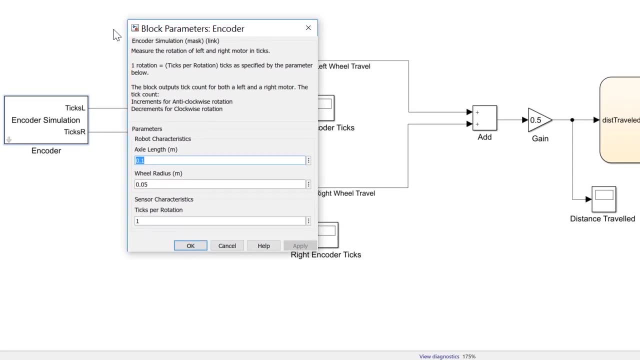 And double click on the encoder block to set up the encoder block parameters. Setting up these parameters will help it mimic a real-world encoder. In our case, we can set it to the variables axillength, Vlar and ticksperrotation. 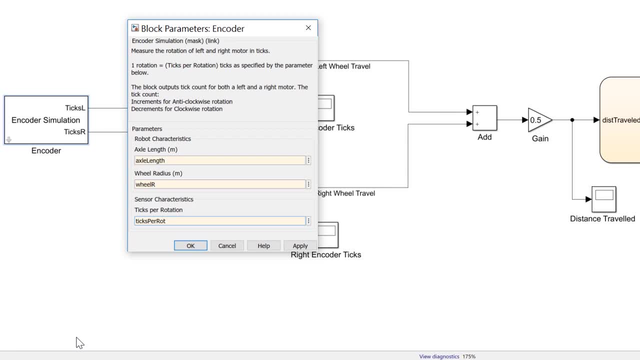 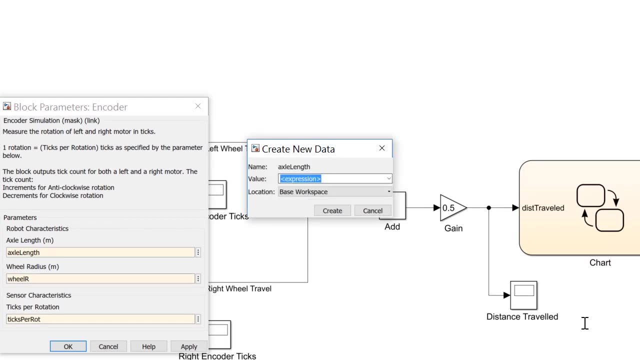 This is the first time we are specifying the axillength variable. So let's create the variable by clicking on the ellipsis here and creating the variable, And let's set its value to be 0.28.. And let's create. And now, 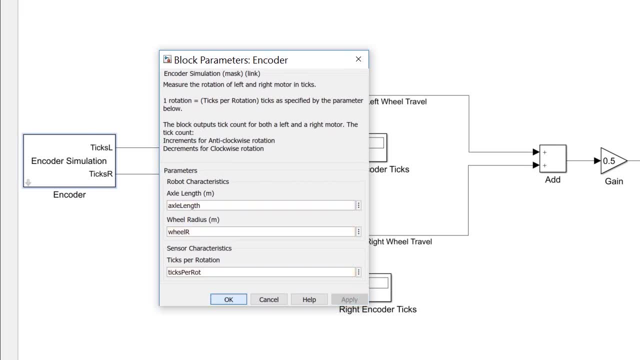 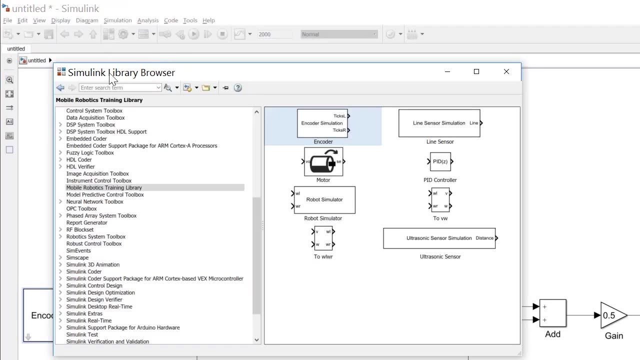 let's hit apply to save the changes. Now, going back to the model for the output, let's use our robot simulator block that is in the mobile robotics training library. So let's go back to the Simulink library browser and choose the robot simulator block and add it to our model. 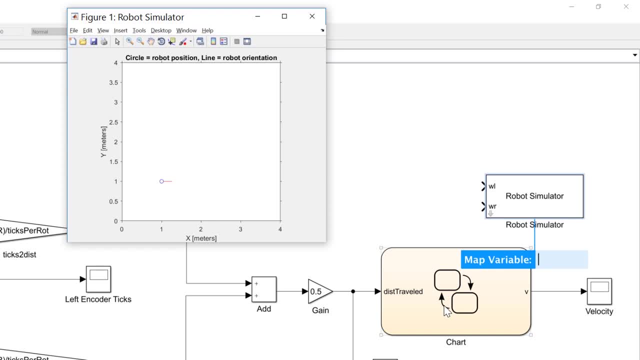 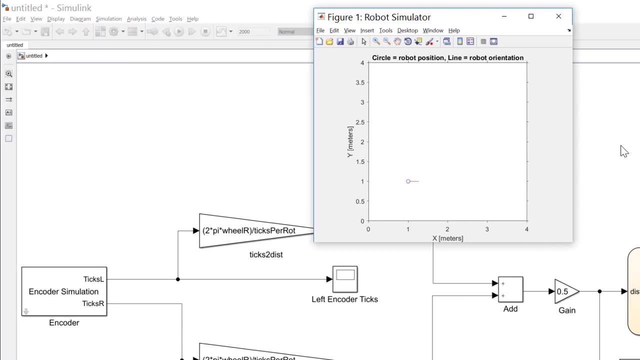 Note that the simulator takes in left and right wheel angular velocities as inputs. The output of the state flow chart, however, is a linear velocity. We need to convert this to wheel velocities. To do so, let's go back to the training library and bring in the utility block 2, omega L, omega R. So let's go back to the training library. 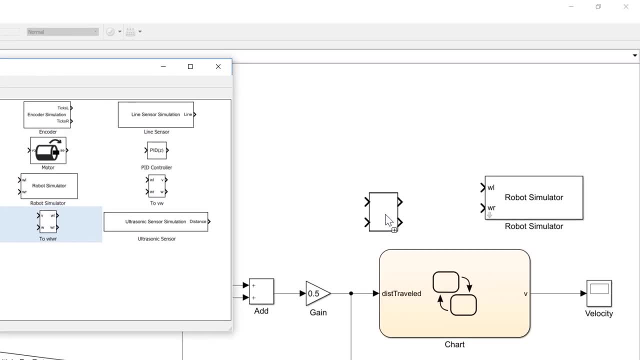 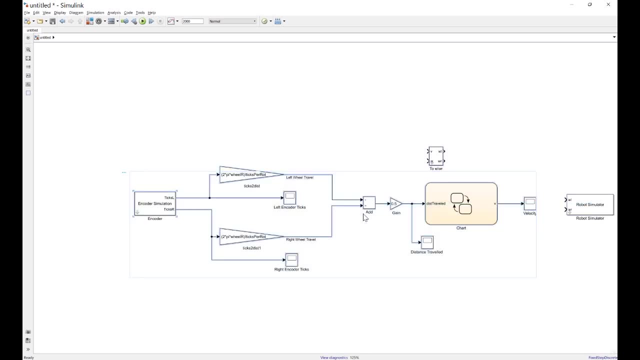 and pick up the utility block 2, omega L, omega R. Let's just resize our model. And now let's connect the output of the state flow chart to the model. Now let's connect the output of the state flow chart to the model. 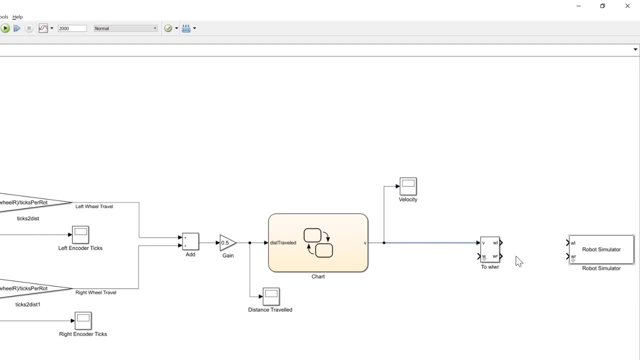 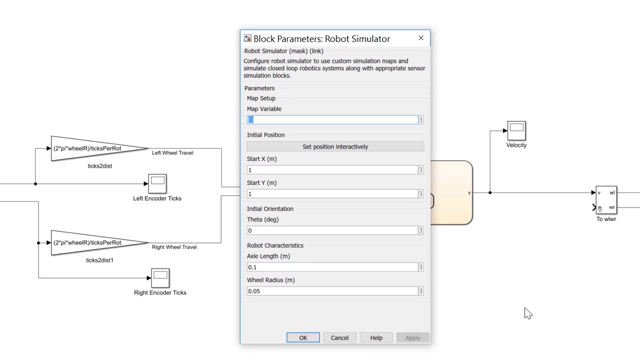 the utility block and the output of the utility block to the simulator. Next, we need to double click on the robot simulator block to set up its parameters. The simulator can use a pre-generated map. We will talk about this in a later video. 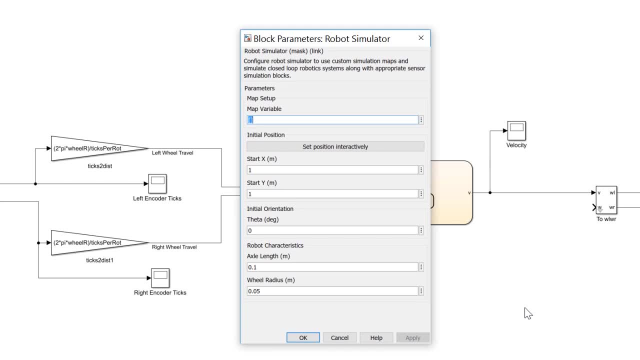 For now let's leave it empty For the starting position. let's start it at a location 1 comma 1, with 0 degrees as the initial orientation And finally, let's specify the physical characteristics here. So let's specify axle length and wheel radius. 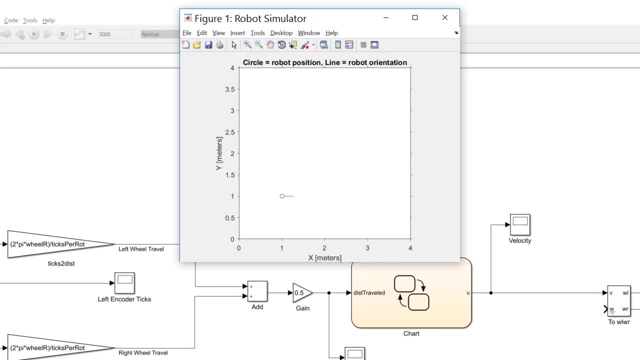 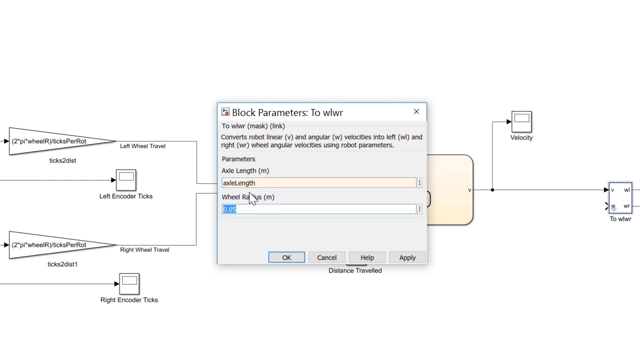 Select OK. We see a window that shows the robot with its orientation starting at 1 comma 1.. Let's go back to the model and double click on the 2 omega L, omega R block to set up its parameters. So axle length again, and wheel radius. 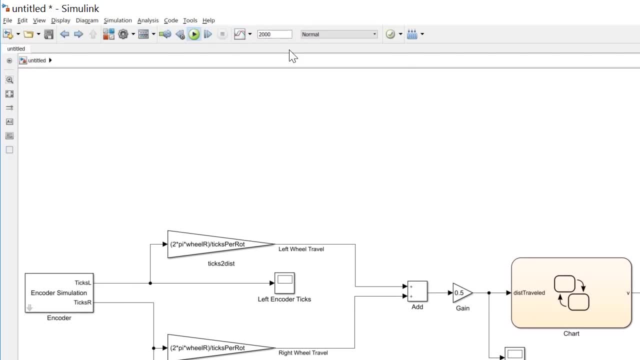 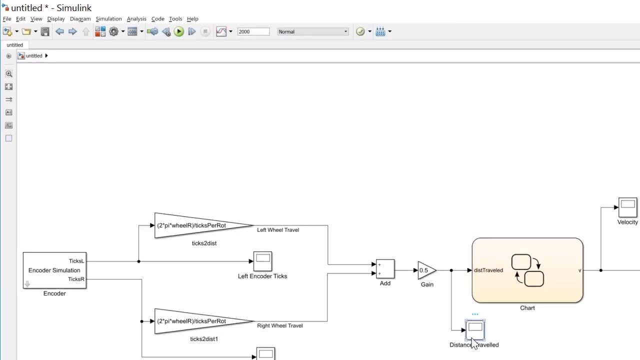 And let's hit OK. Now let's run the model. We see that the robot is moving in a horizontal direction and only stops when the robot is near the 2 meter mark. Now let's take a look at the distance travel scope. We see that it. 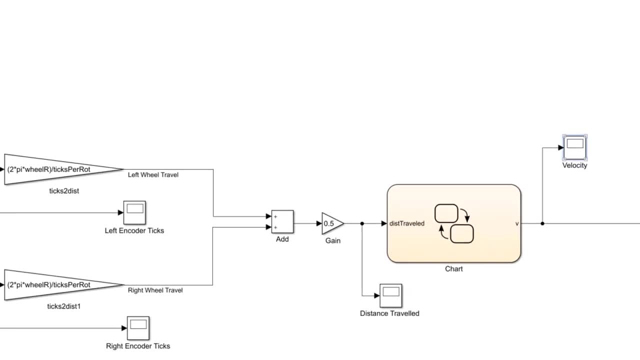 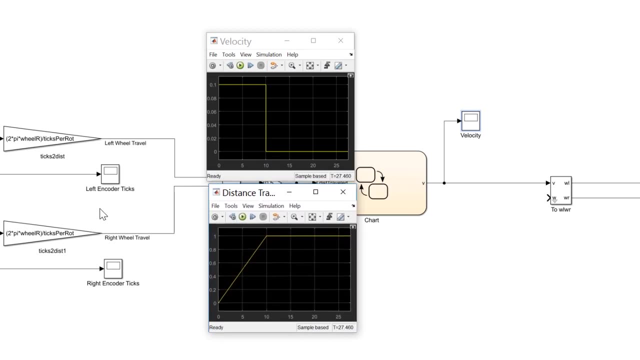 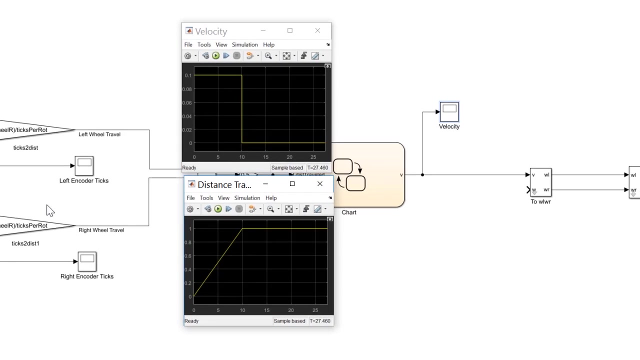 tapers off near the 1 meter mark. Opening the velocity scope and comparing it with the distance scope, we can see that the velocity has dropped to 0 as soon as the distance of 1 meter is reached. So, all in all, we have simulated a closed loop system with the help of the simulated sensors. 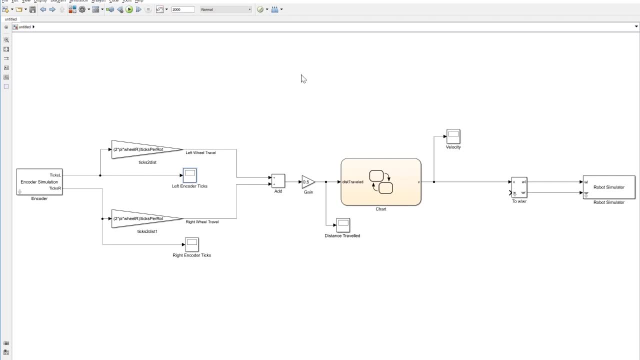 So now that we have seen our algorithm in simulation, we need to see this in action on a hardware platform. Hardware support can be extended in Simulink by downloading and installing additional support packages To see this. let's go back to MATLAB. 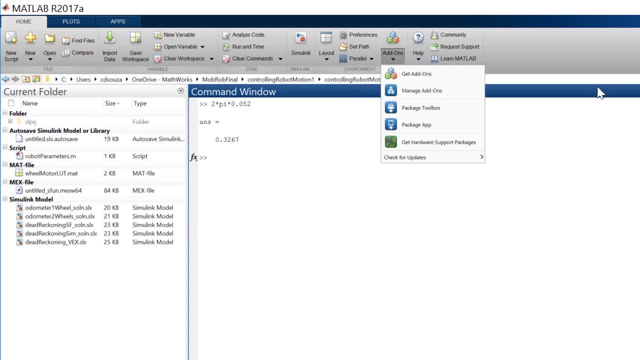 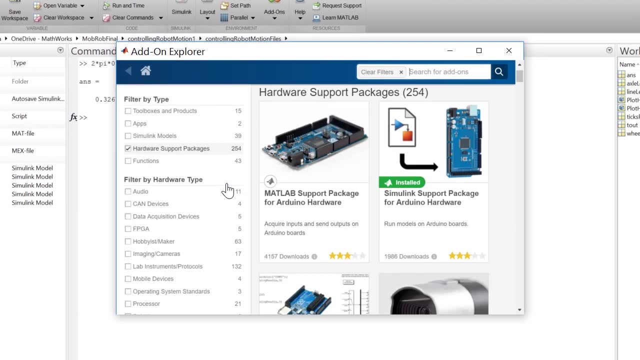 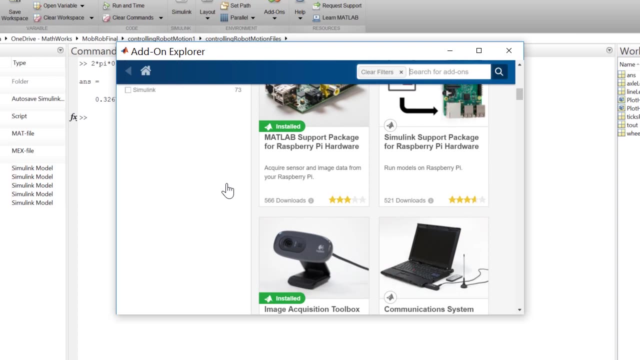 In the MATLAB tool strip, use the add-ons menu and click on the get hardware support packages option. As you can see here, several platforms such as the Arduino, the Raspberry Pi and the Lego are supported. In our examples, we are going to use the VEX microcontroller platform. 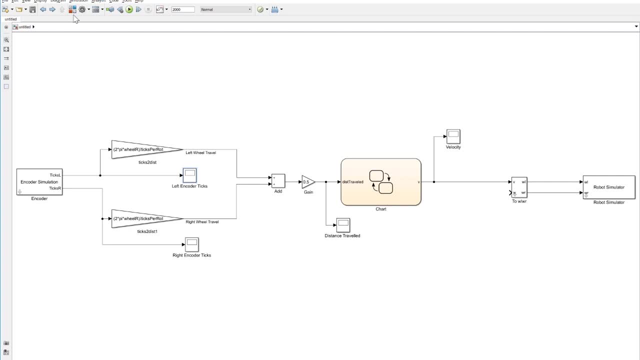 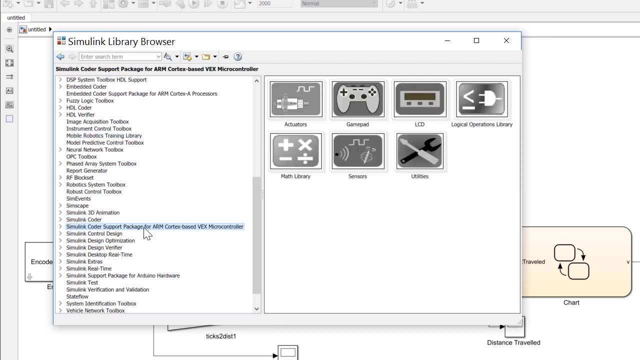 So let's look at this library in Simulink. In the Simulink library browser, scroll down to the Simulink coder support package for ARM Cortex-based VEX microcontroller. This is what you would get when you install a hardware support packages. We see several blocks. 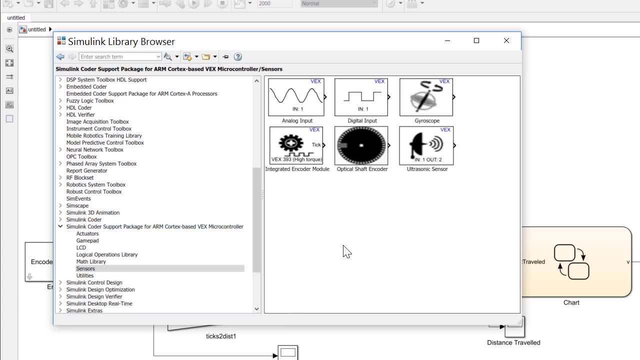 Let's dig into the simulation. We can see encoders, ultrasonic sensors, etc. Remember the blocks that we used in the training library are for simulation. These blocks can be used to connect to the actual hardware. You can also scroll through the library browser to see another example for hardware support. 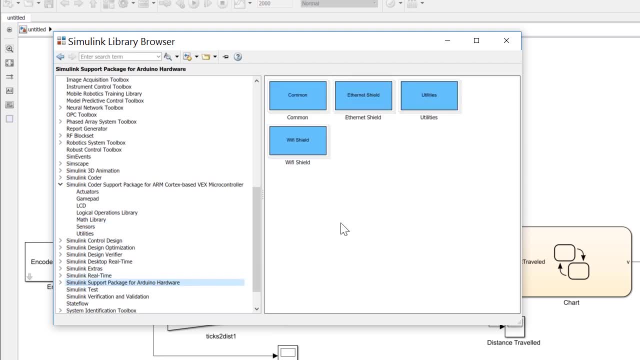 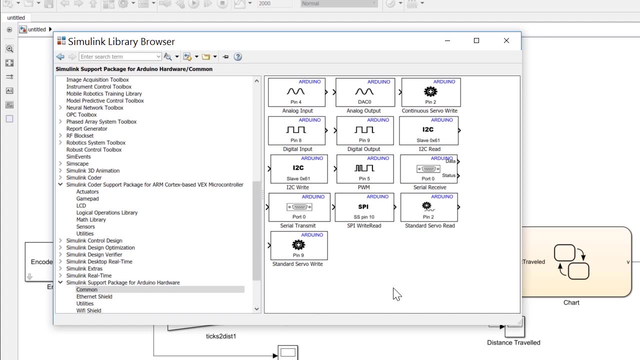 You can see the Simulink support package for the Arduino hardware. We can see similar blocks here, Even though we are using the VEX microcontroller platform. we can see that the hardware support packages are also supported Even though we are using the VEX platform in our examples. 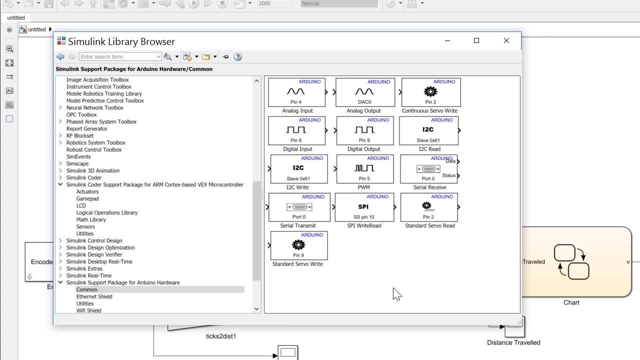 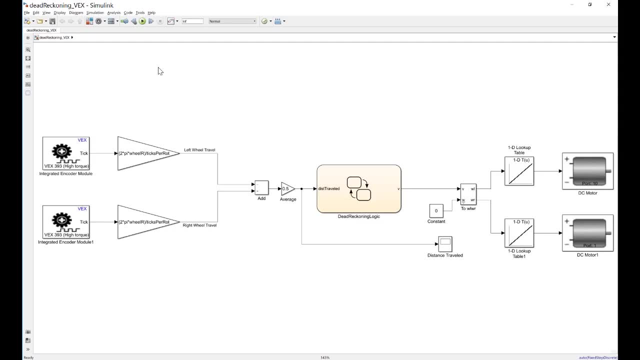 the design methodology can be extended to other platforms as well. Let's go back to MATLAB and open the model deadreckoning underscore VEX, which is right here. Here we see the blocks from the VEX support package, namely the encoders and the motors that have replaced our simulation blocks. 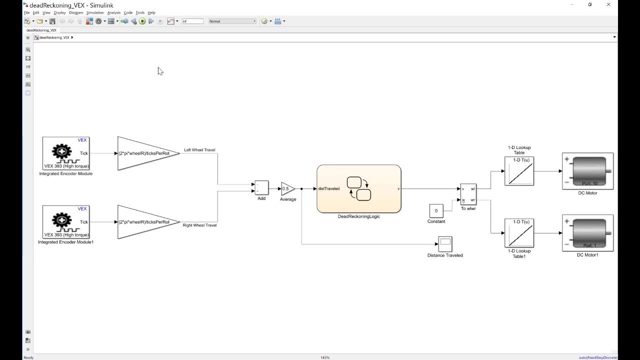 There is another change in this model. The motor takes in a voltage value, However the output here is the angular velocity. However, the output here is the angular velocity, However, the output here is the angular velocity, So we need a mapping between these two quantities. 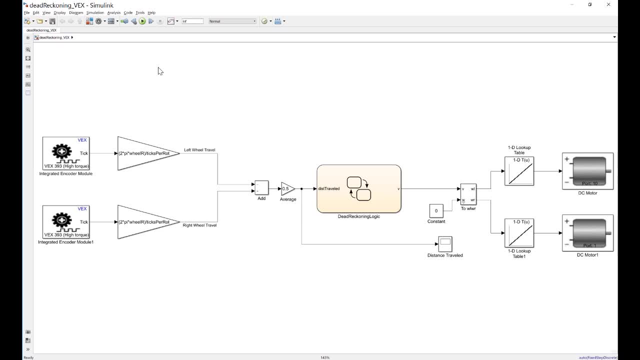 We use a lookup table block to represent the speed characteristics for the motor. Please look at the links in the resources section to get more information on how to use this block. If you are interested in how to run this model on the hardware, we have relevant links in the same place as well. 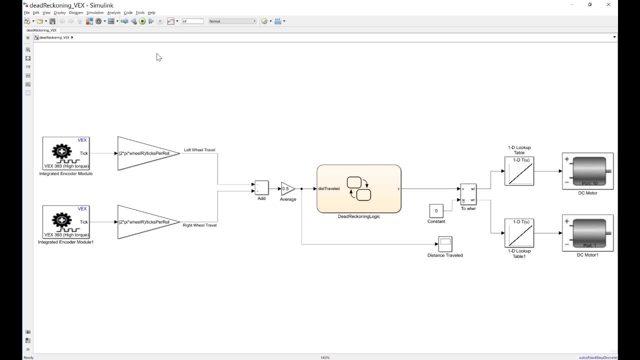 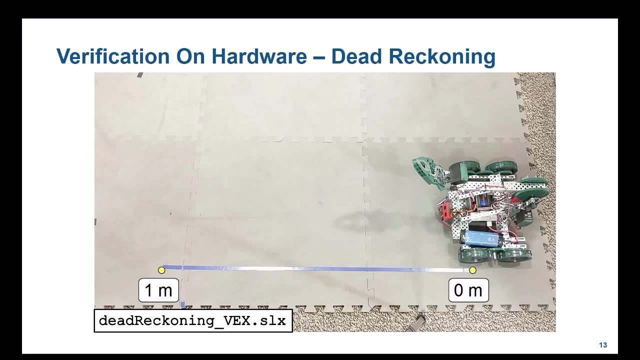 For now, let's go back to the presentation and see how this model worked on the hardware. Here we see a robot lined up at the start of a blue line. The end of the blue line signifies the one meter mark. Let's see how our logic performs on the hardware. 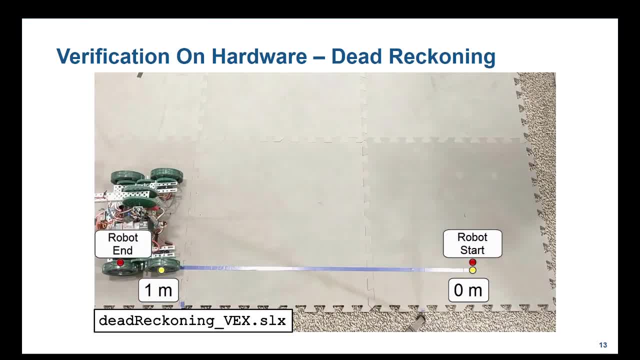 This was the result we achieved. We can see that the robot ends up way beyond the one meter mark signified by the red dot near the end of the line. So why did our simulation say we will reach one meter exactly, but the hardware shows a different result? 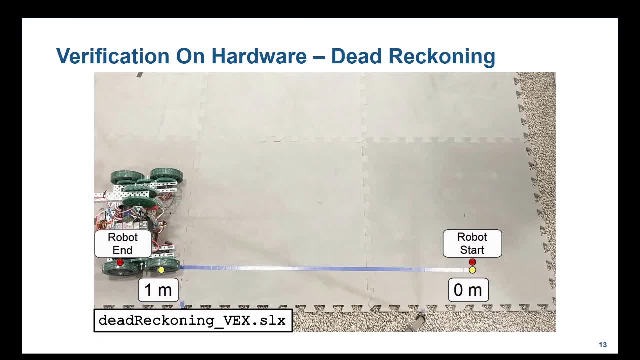 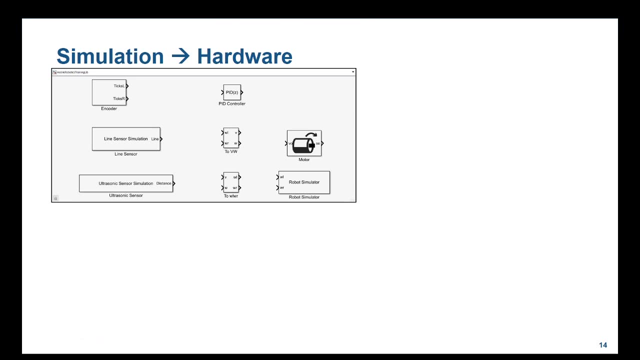 How do we get the robot to reach one meter more accurately? These are some of the questions we will answer in the next video, while talking about PID controllers. To recap the high-level workflow, we used the mobile robotics training library to design our algorithm in Simulink. We then used one of the hardware support packages available. 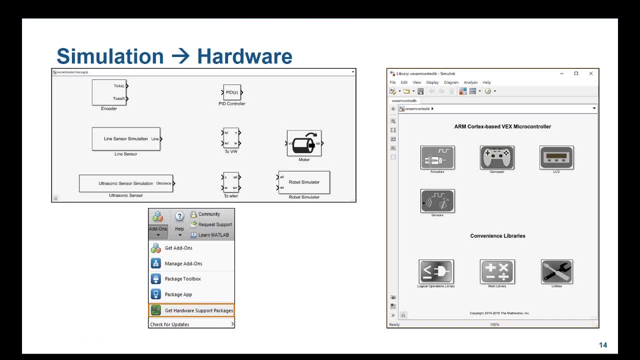 namely the VEX platform, to replace the simulation blocks with the hardware blocks to test it on the hardware. Even though we are using the VEX platform in our examples, this design methodology can be extended to other platforms such as the Lego, Arduino, Raspberry Pi. 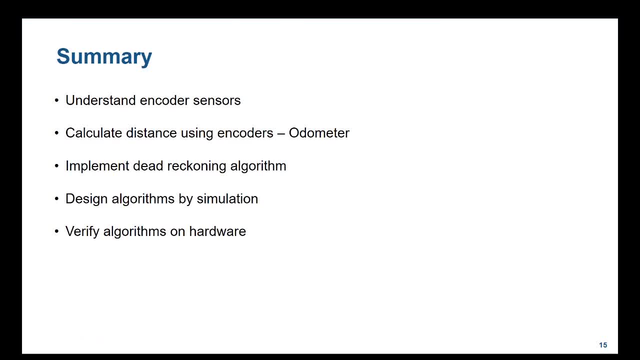 etc. In summary, we talked about the basics of encoder sensors and how they can be used to compute the number of wheeled robots. We also talked about the basics of encoder sensors and how they can be used to compute the number of wheeled robots. 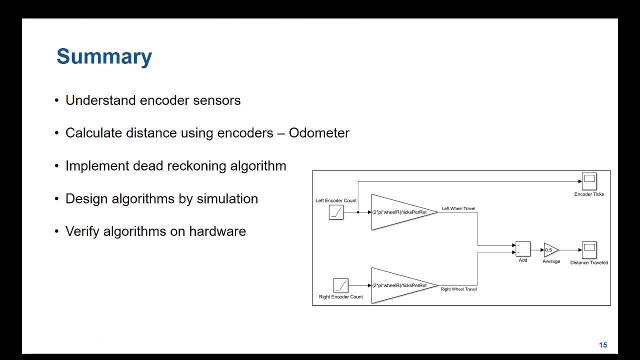 We also talked about the basics of encoder sensors and how they can be used to compute the number of wheeled robots. We then calculated the distance using encoders. We used this example to introduce Simulink modeling techniques. By the end of this, we had a Simulink model that could be used to calculate distance traveled. 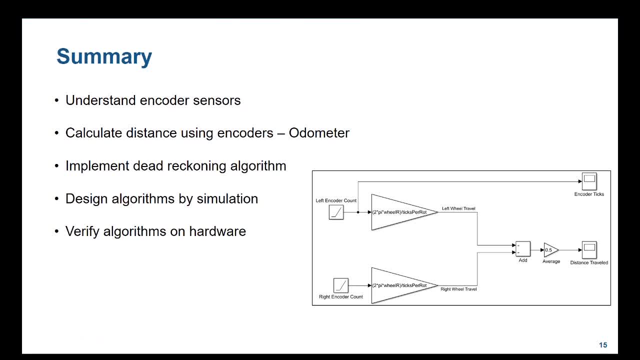 given the number of encoder ticks, or vice versa. We then implemented a dead reckoning algorithm. We used this example to introduce stateflow modeling techniques. By the end of this, we had a model that could verify an algorithm with simulated inputs. The next idea was to use a closed-loop simulation to make testing algorithms more efficient.